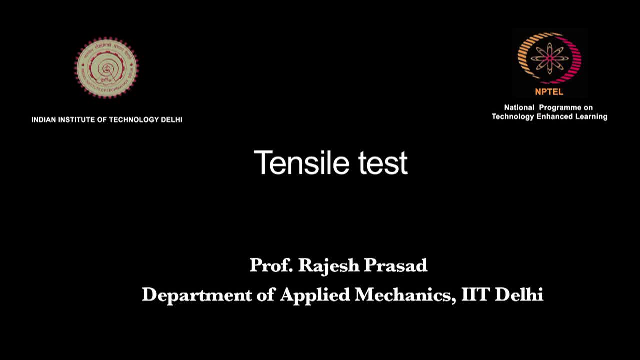 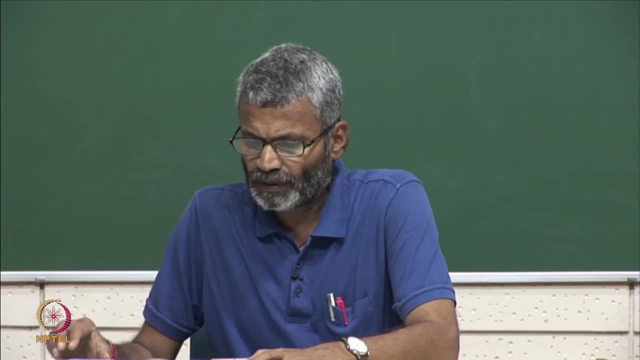 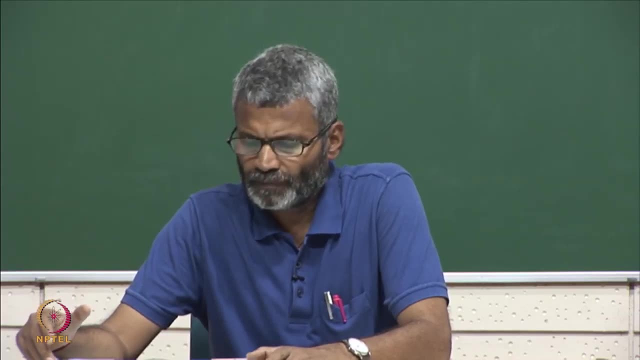 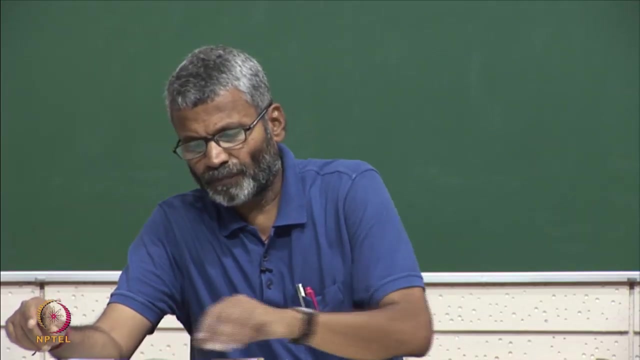 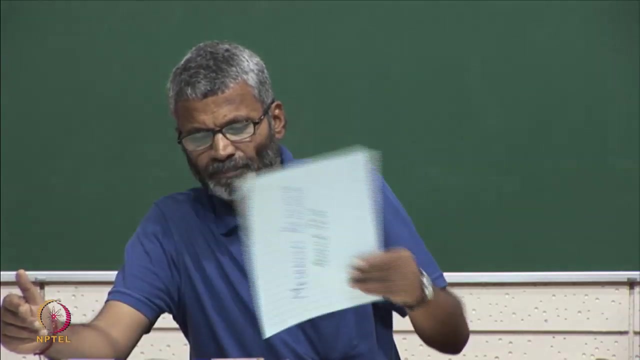 Let us now discuss the mechanical behavior of materials. One of the quick way and easy way to find mechanical behavior and a starting point is usually the tensile test. It is a simple test which gives us various mechanical behavior parameters or mechanical properties of material. So let us look at this simple test. A uniaxial tensile test is usually done. 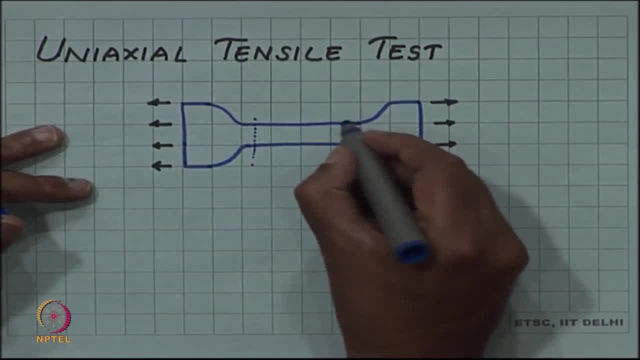 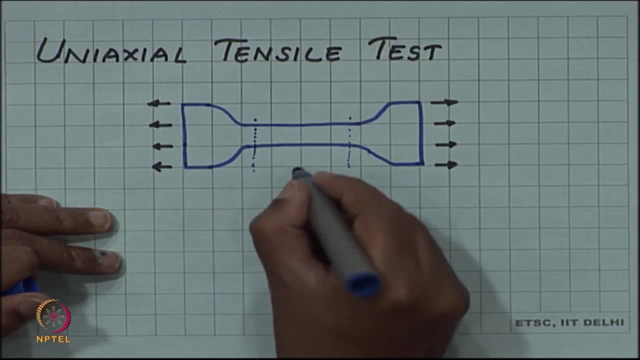 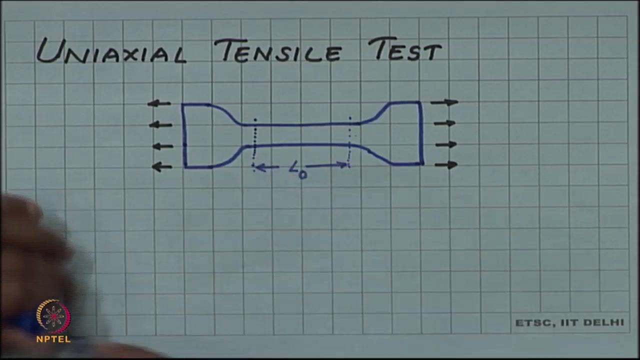 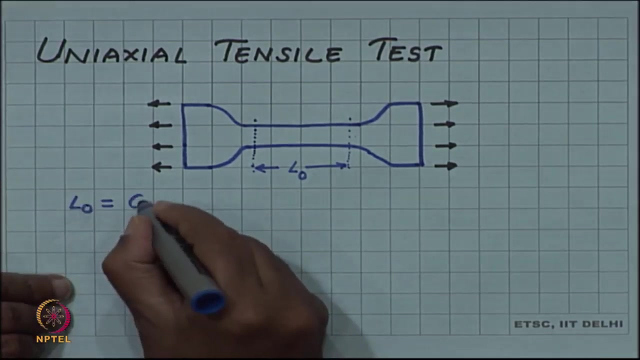 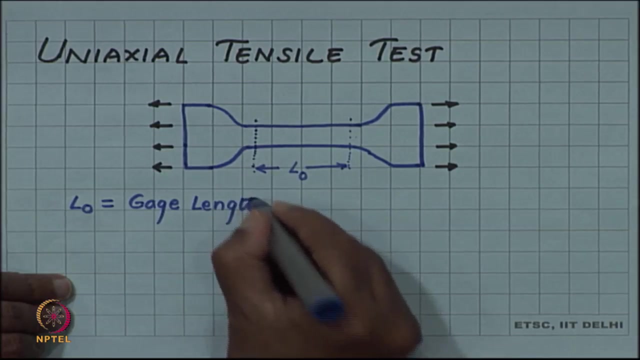 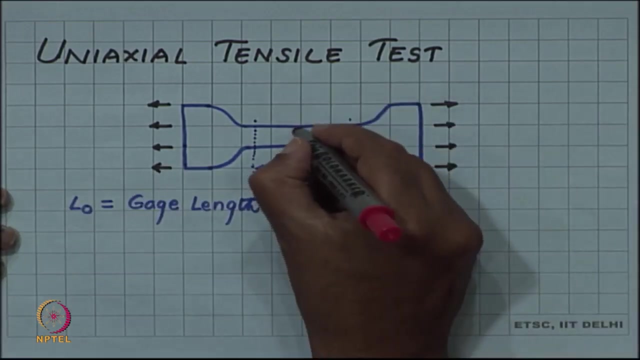 on a sample of this kind of shape, where this central portion is of uniform cross section and the length of that portion is called the gaze length. So this is the uniaxial tensile test, This is the gaze length, and gaze length has a uniform circular or rectangular cross section. 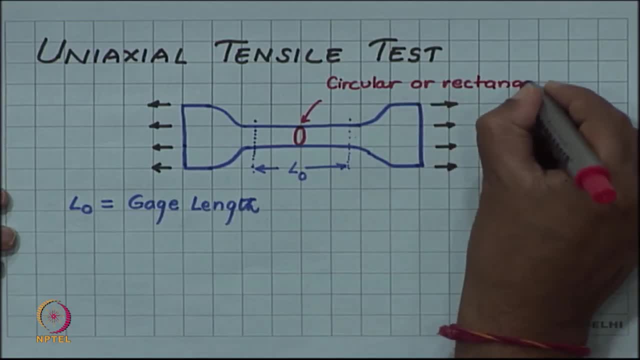 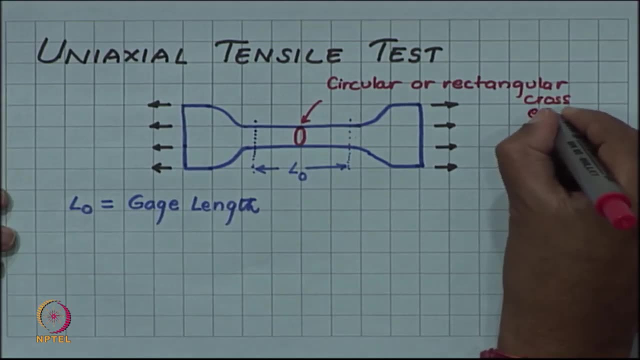 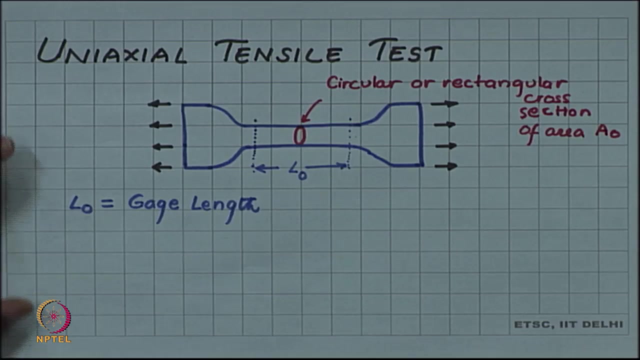 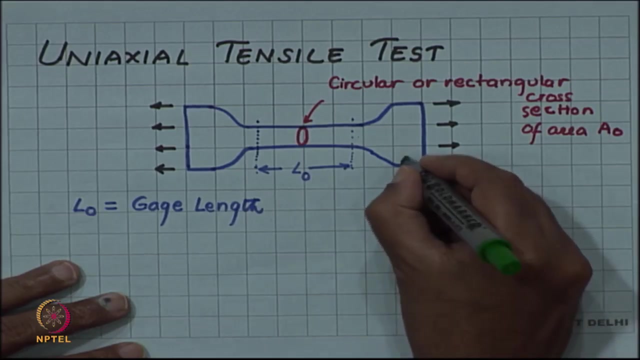 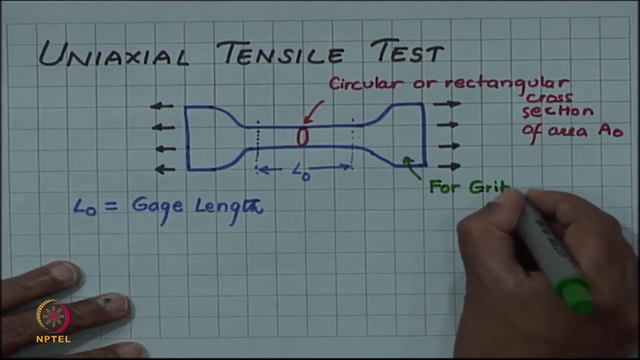 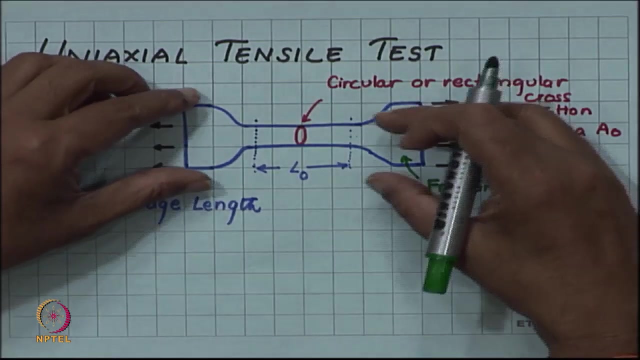 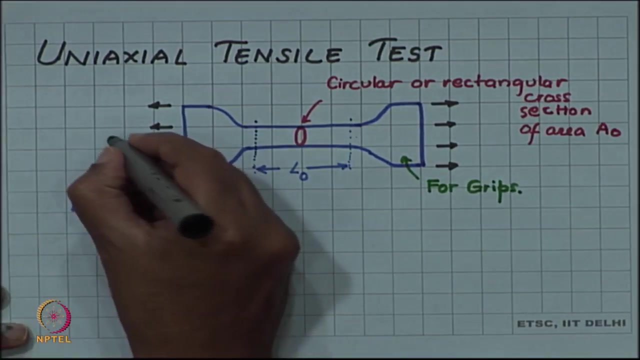 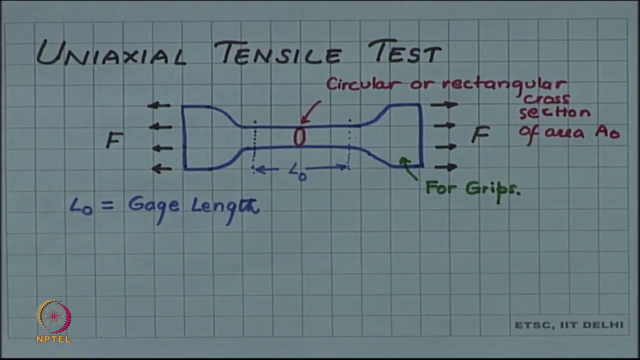 Of area A naught. the larger portion here at the ends is for gripping the sample. So this is for grips. Now such a sample is held in a tensile machine, is gripped at the two ends and is then pulled under a force. So you apply a force F and pull the specimen. 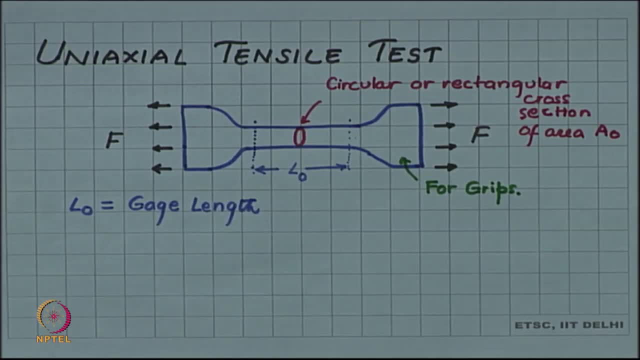 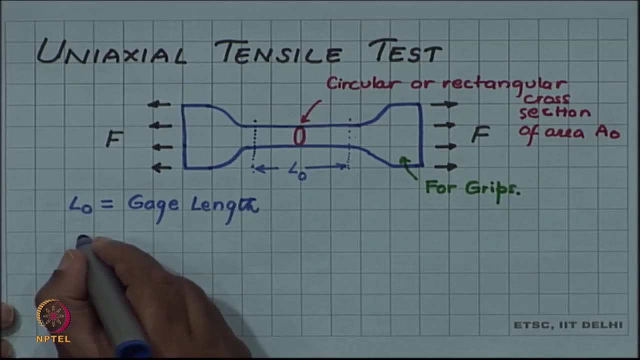 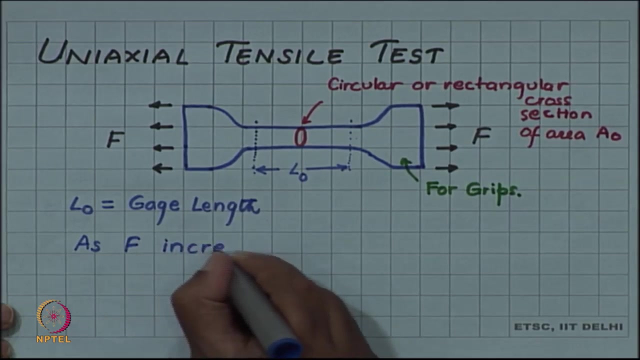 As you pull the specimen, the specimen will elongate, and as the force will increase, the sample will elongate. So as F increases, length changes. So this is the uniaxial tensile test. So this is the uniaxial tensile test. So this is the uniaxial tensile test. So this 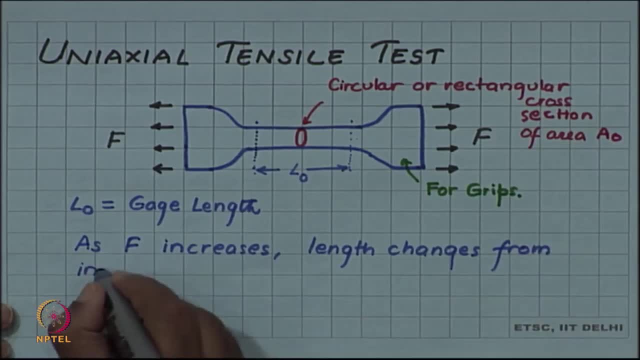 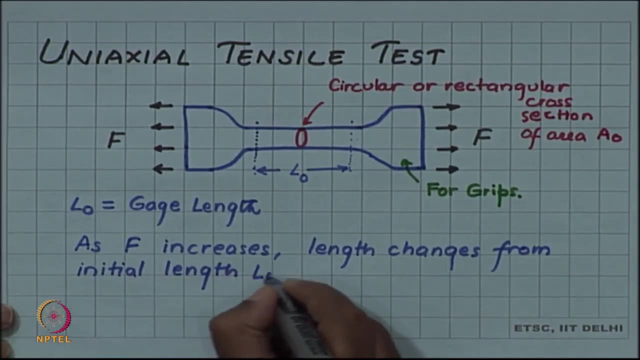 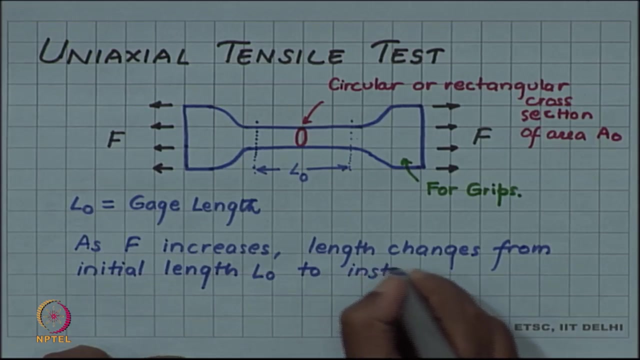 is from initial length L naught to instantaneous length L. So this is the uniaxial tensile test. So that was done earlier. So what about the mass and activity, doncra, sir? thus? So that is a total mass of manga and a mustard hte. The mass of this sample is Nadol. Now, traditionally the mass, ha, rgery and the mass is equal to the mass of the sample, but this is just to show that the size is. I not consider the size. if the sum of the two paper has been multiplied to double, that is 7.1, so will take the last moment to measure the millimetre. 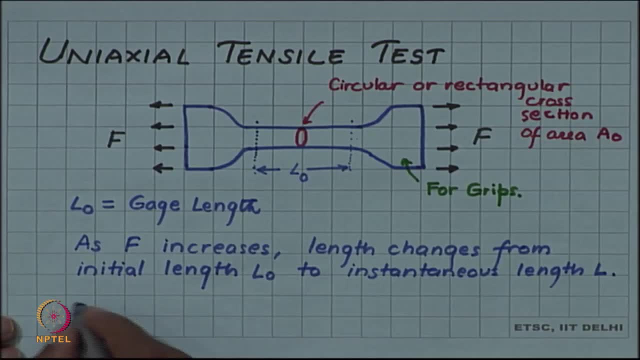 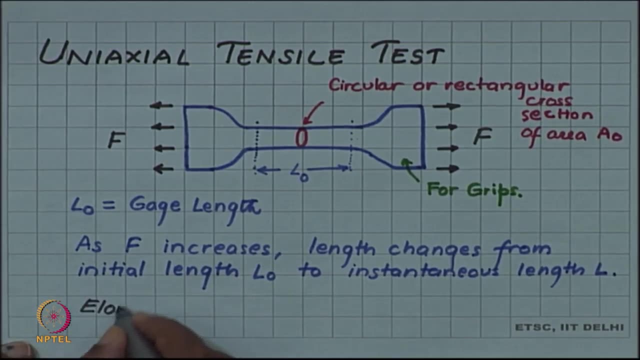 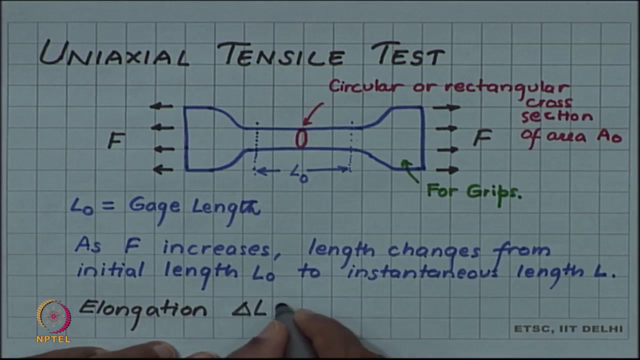 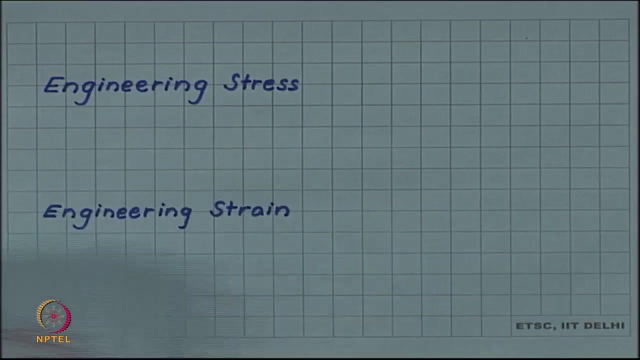 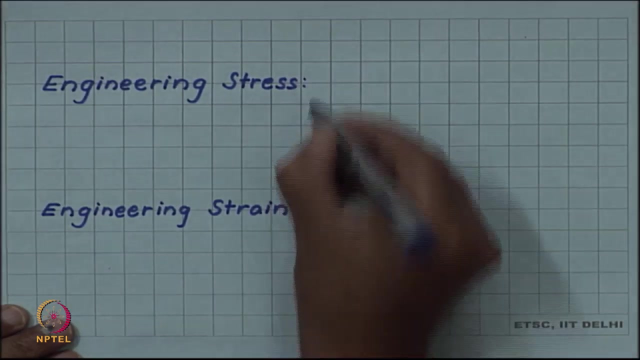 So the change in length is called the elongation of the specimen elongation symbol. delta L is given by L minus L naught. So this is a simple uniaxial tensile test. The uniaxial tensile test, the variables, instead of force and elongation, are taken to be engineering. 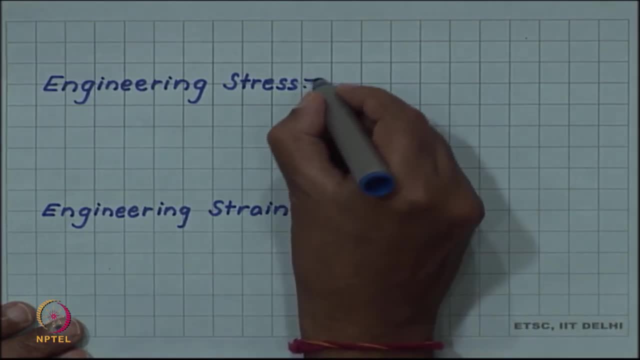 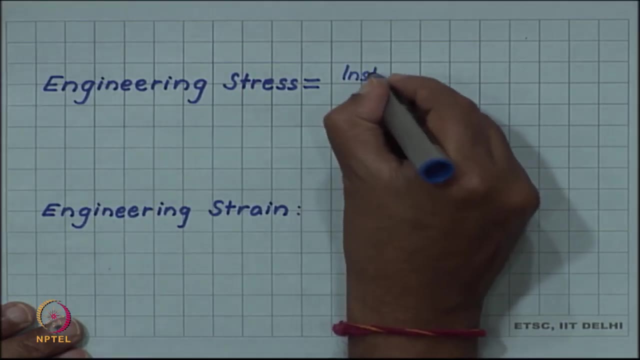 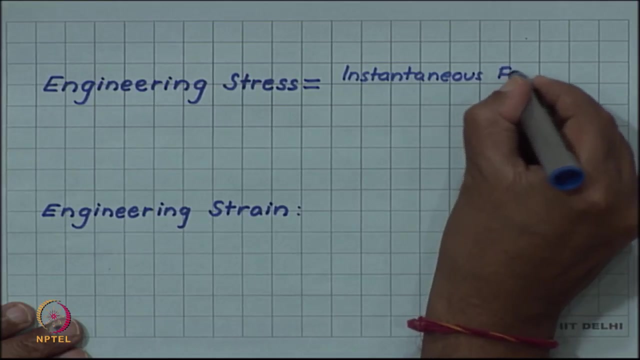 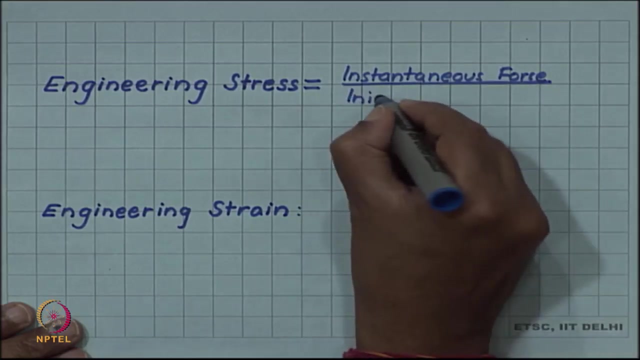 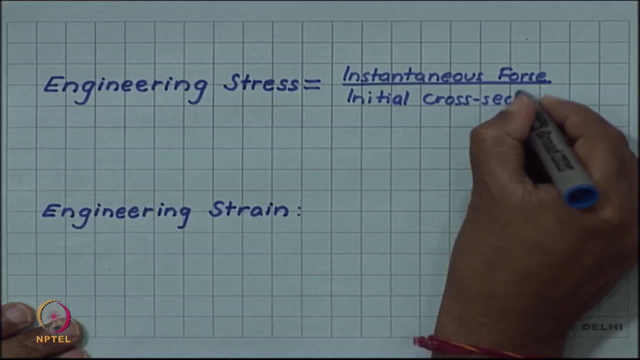 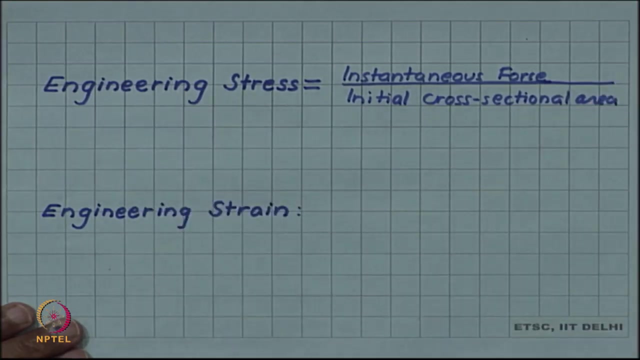 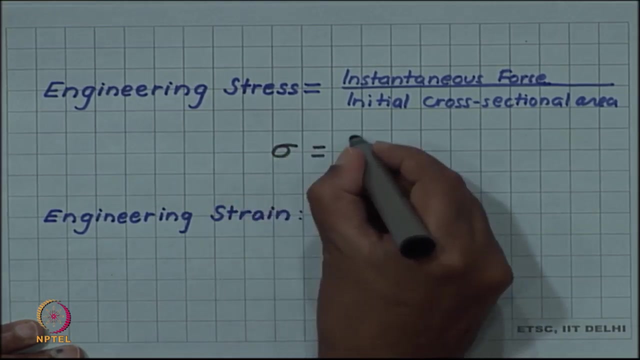 stress and engineering strain. We define the engineering stress as the stress of the specimen, instantaneous force by initial cross sectional air. So in factwheel strength is given depositive strength. So this work will be来11 אMus standard area, A common symbol for engineering. a stress is sigma for force. we use f and for initial 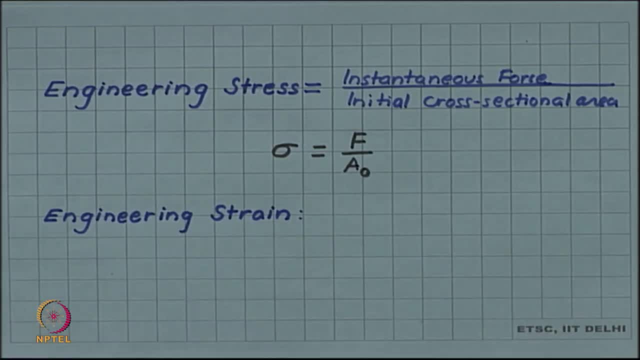 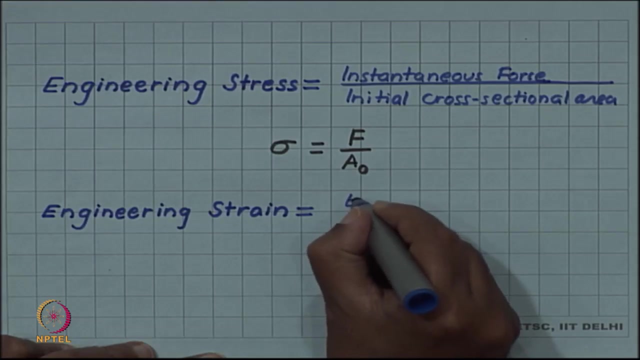 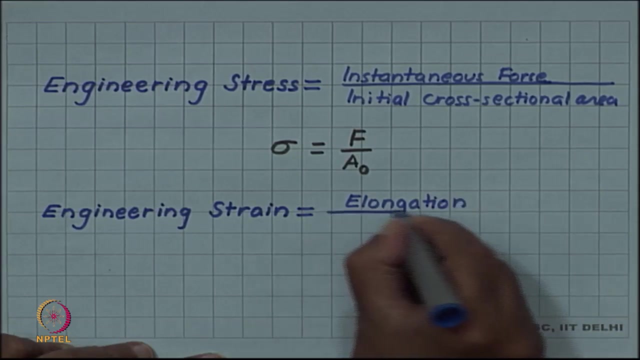 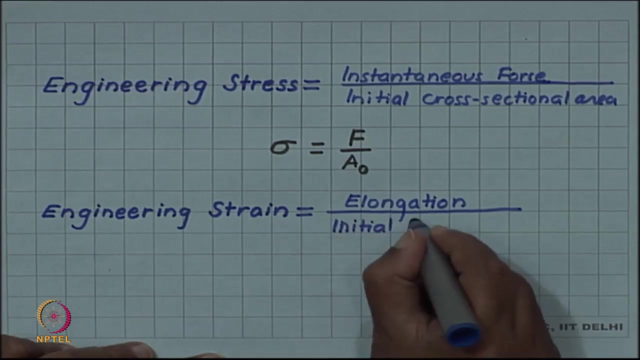 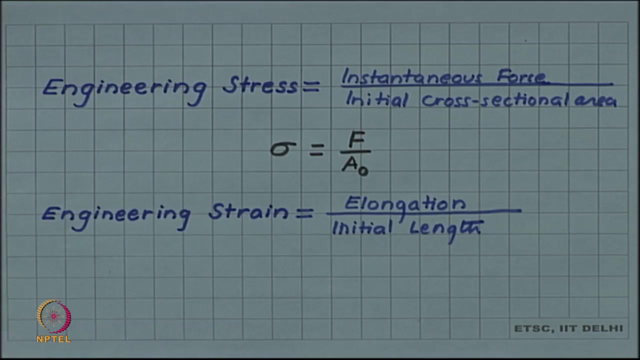 cross sectional area. a naught, So we have sigma, is equal to f by a naught. For engineering a strain, we define elongation divided by initial length or the gauge length. So we have the symbol for engineering a stress is sigma. for force, we use f by a naught, So we have 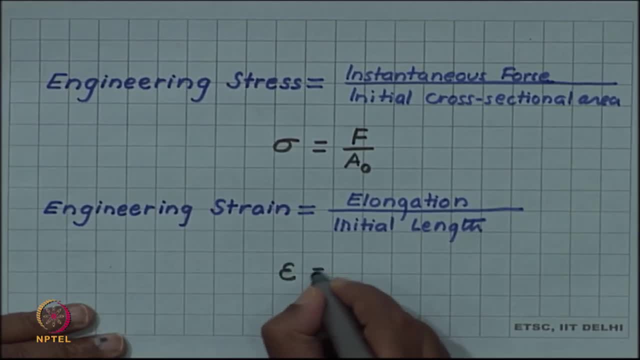 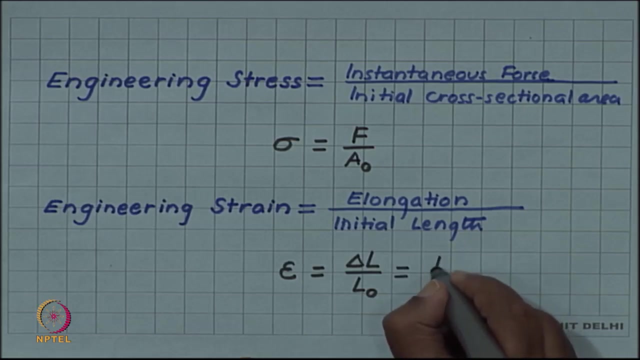 sigma for engineering. a stress is sigma for force. we use f by a naught, So we have engineering. a stress is epsilon, which is change in length divided by the initial gauge length. or you can write: l minus l naught by l naught, l by l naught minus 1.. 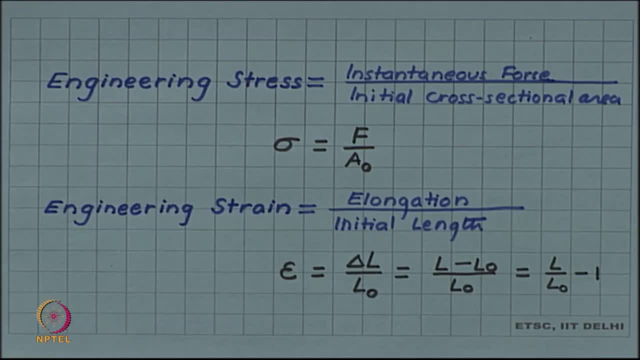 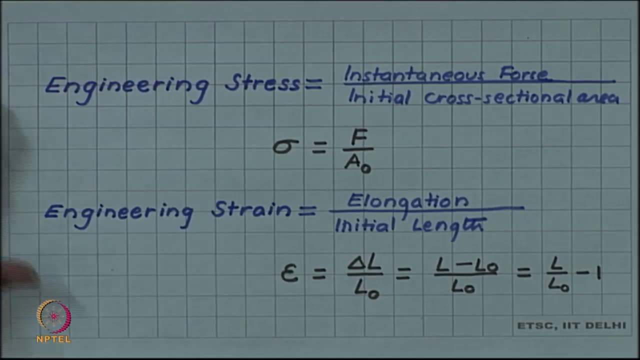 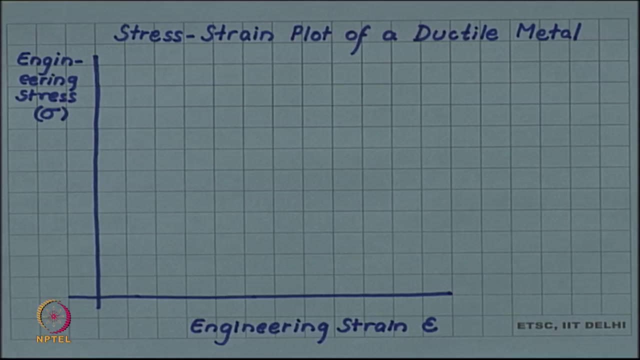 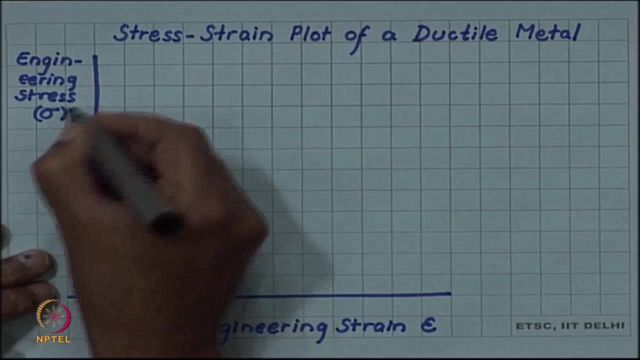 So the result of the uniaxial tensile test is presented in terms of a plot of engineering a stress versus engineering a strain. So the y axis is taken to be the engineering a stress, the x axis the engineering a strain. You have seen that the engineering a stress. 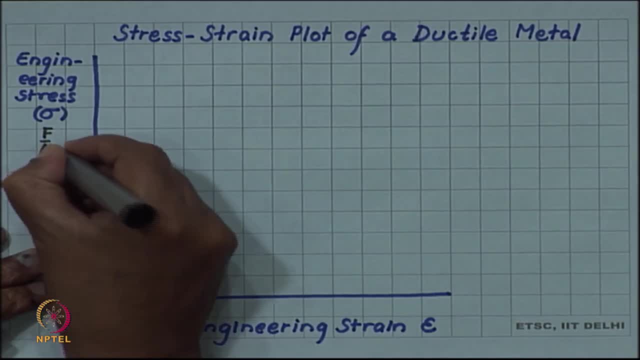 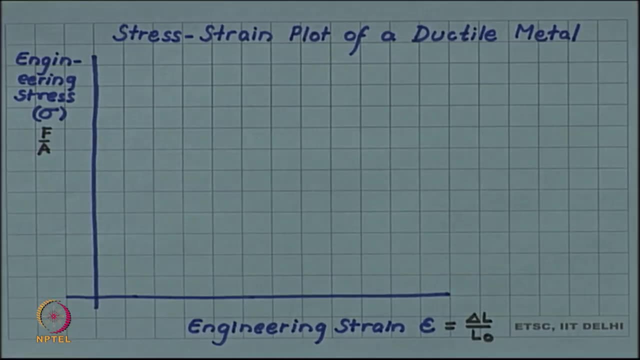 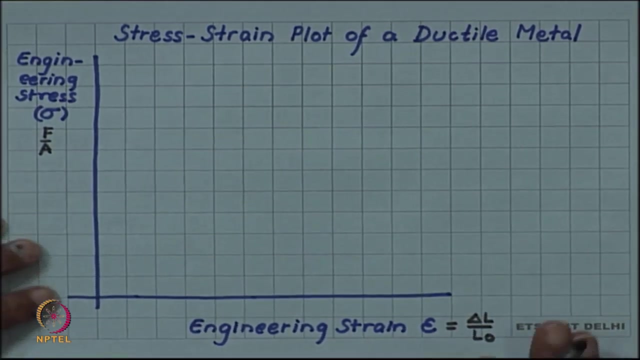 is f by a and engineering a strain is f by a and engineering a strain is f by a. So the g isimo strain is deletile by l naught. so what the result looks like. of course the result depends upon material to material and it can vary a lot if the material type is. 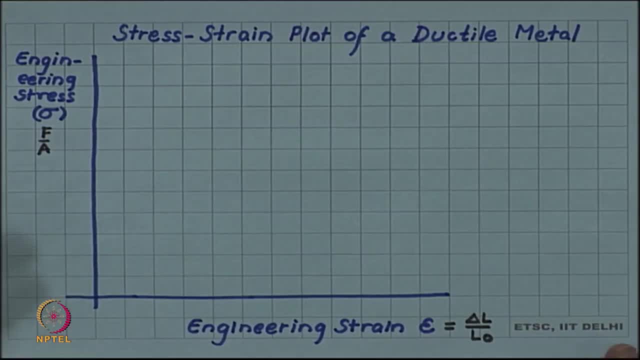 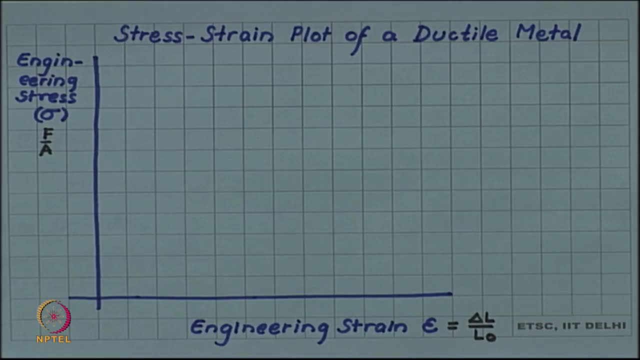 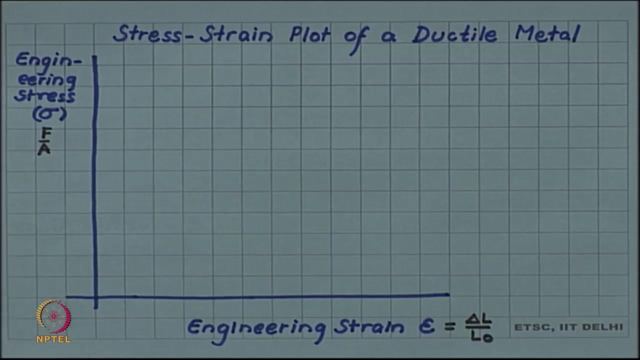 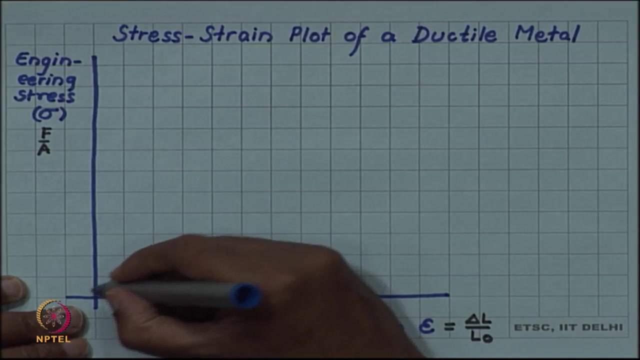 very, very different. For example, metal will show a very different kind of stress strain curve than a polymer or a rubber or a ceramic. So let us look at to begin with, the stress strain plot for a ductile metal. So initially, as the material is being deformed, remember, 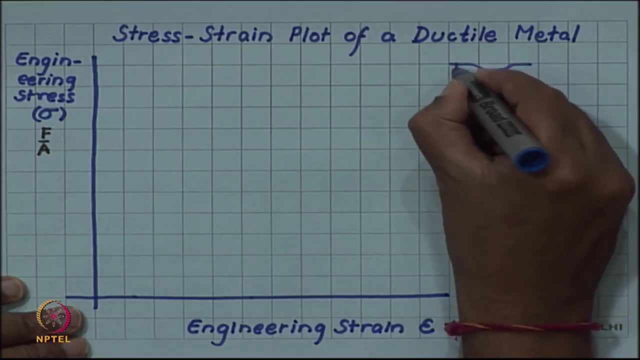 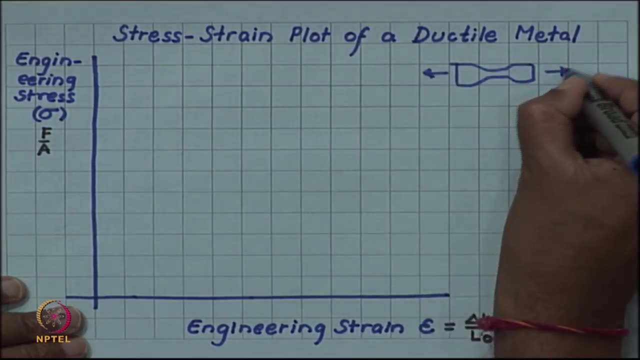 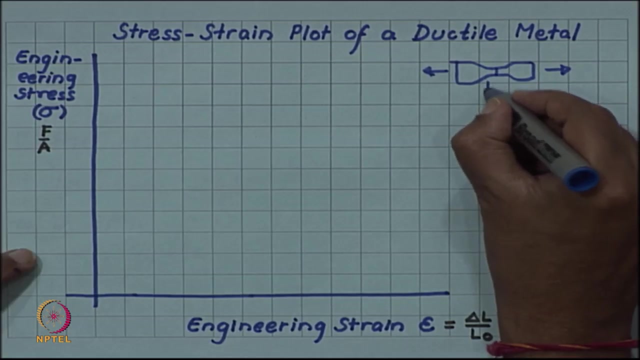 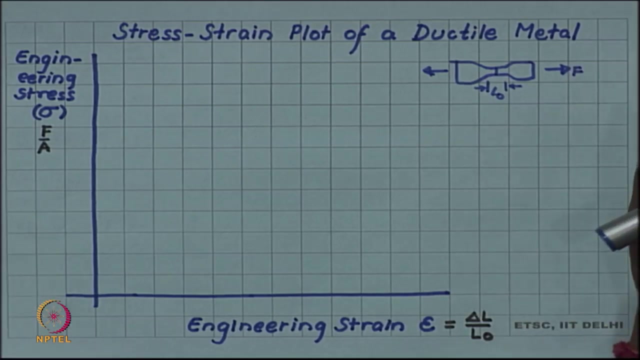 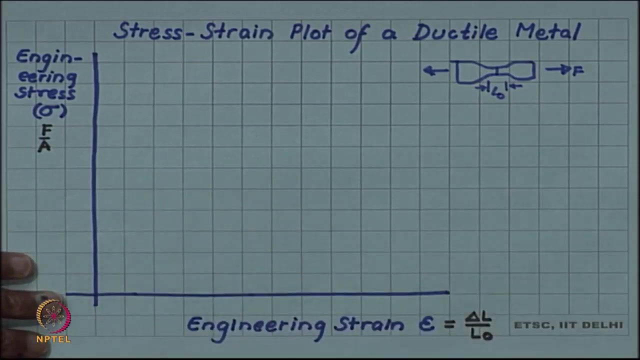 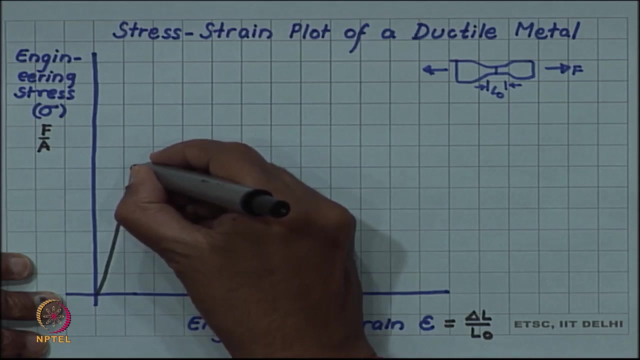 you have a test specimen which is being deformed under load and you are plotting the force divided by the initial cross sectional area and change in length by the initial gauge length. So when we do that we find that for many metals we have an initial straight line portion. 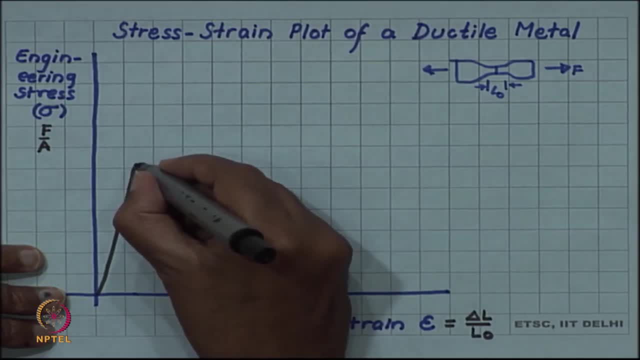 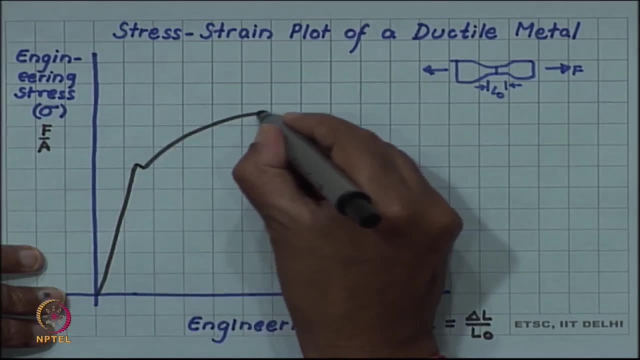 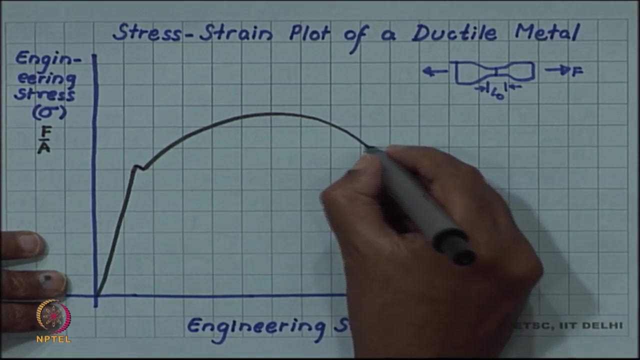 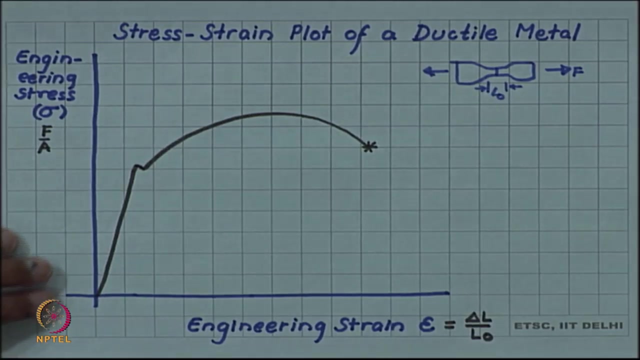 and then we have a cross sectional area, Then there is a nonlinearity develops and the material goes through a maximum load and finally it breaks at some point. This is a typical stress strain plot of a ductile material. This is a typical stress strain plot that, through the analysis of such a plot, many parameters, 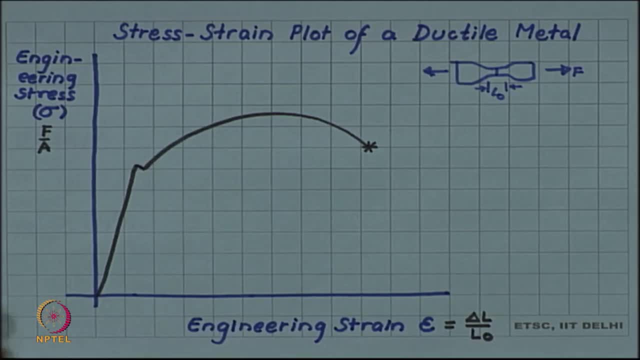 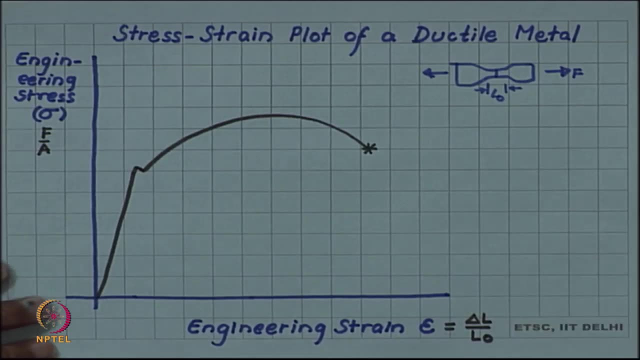 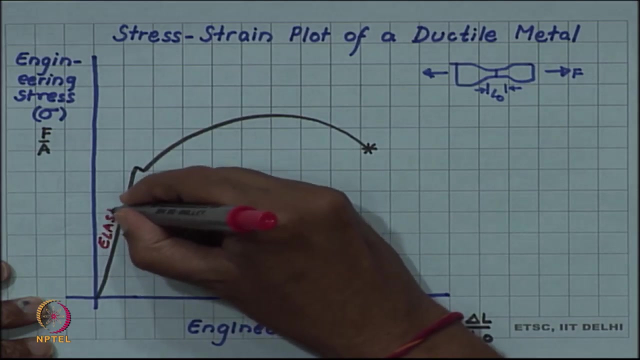 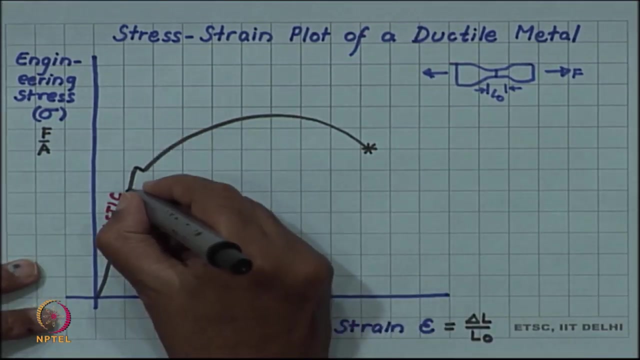 of mechanical interest can be derived. First of all, we see that in the initial portion is linear. this is an elastic portion. That is, if we unloaded the material, if we did not go all the way up to Further deformation, suppose we stop the test here and we unloaded, then the material would. 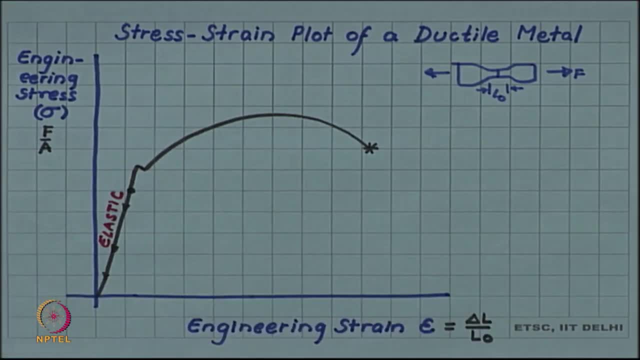 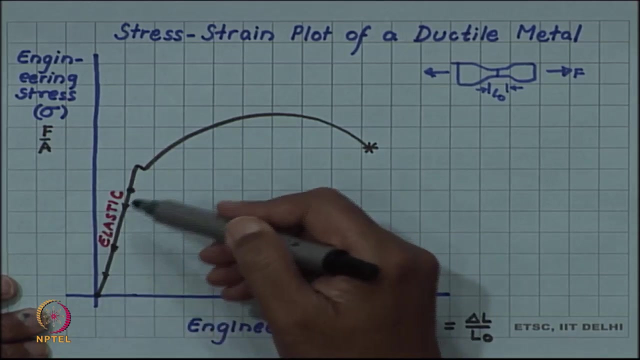 have followed this same line back to the origin and there would have been, at 0 load, there would have been 0 deformation at 0 stress, 0 strain, So material would have come back. So this is a reversible deformation and is an elastic deformation. But if we keep deforming, the 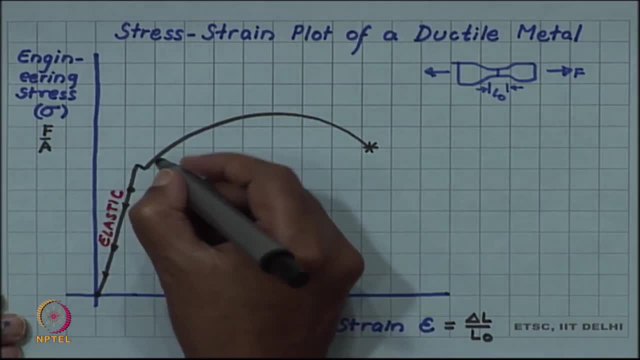 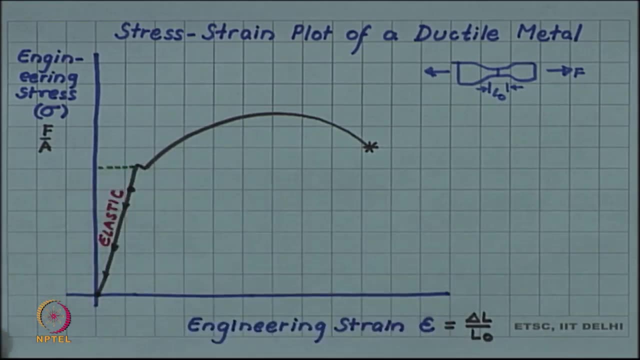 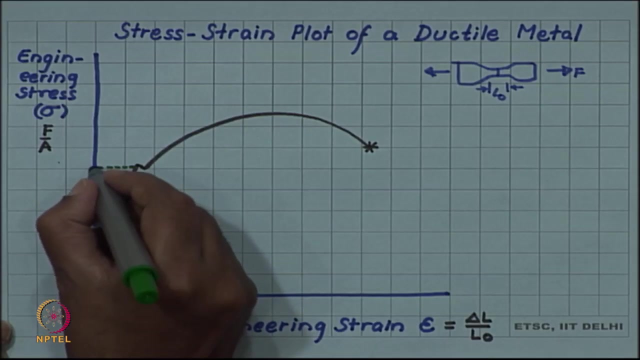 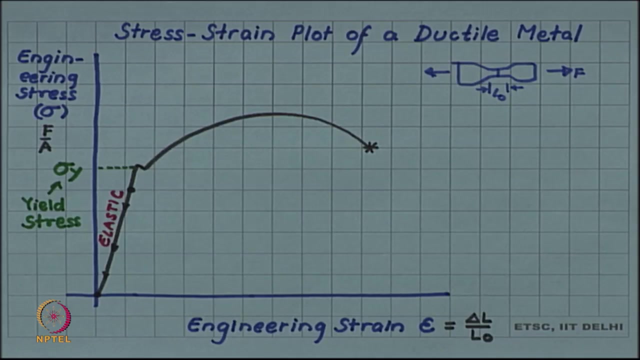 material, the elastic deformation keeps increasing and at some point the material stops being linear and stops being elastic and starts undergoing what is called a plastic deformation. This point, this stress corresponding to this point, is called the yield stress. That is the point where the plastic deformation 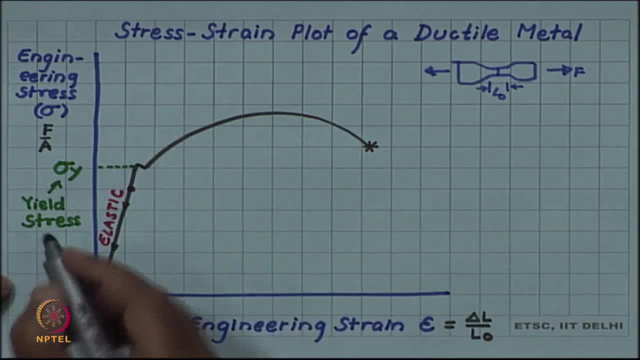 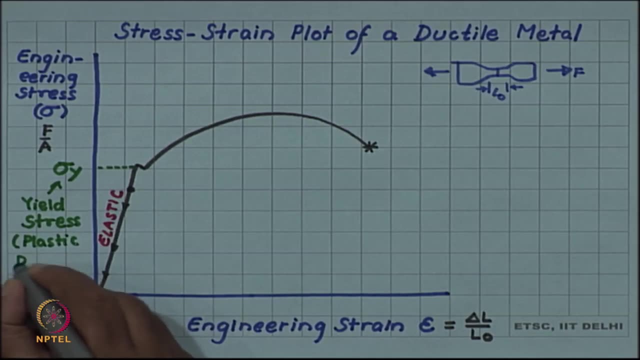 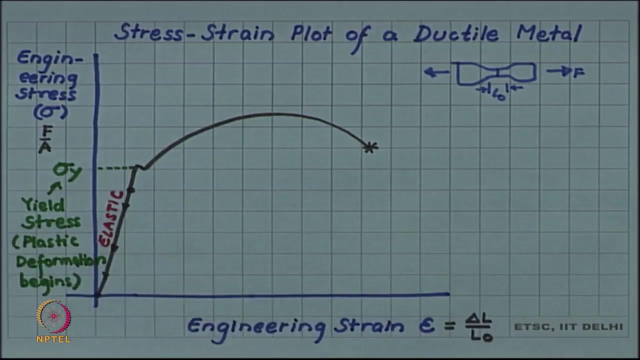 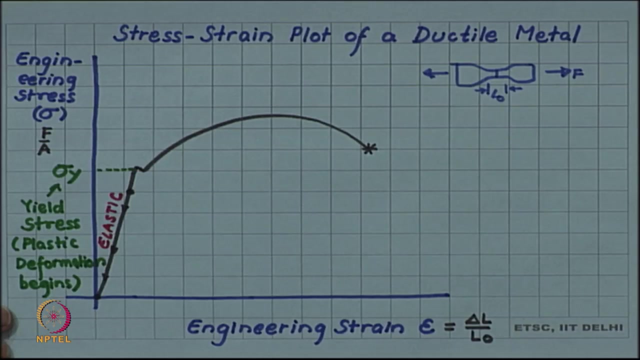 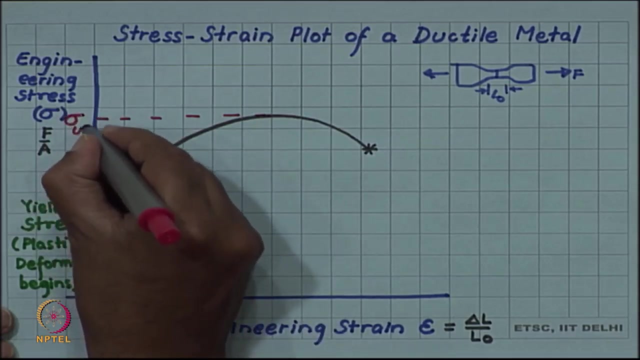 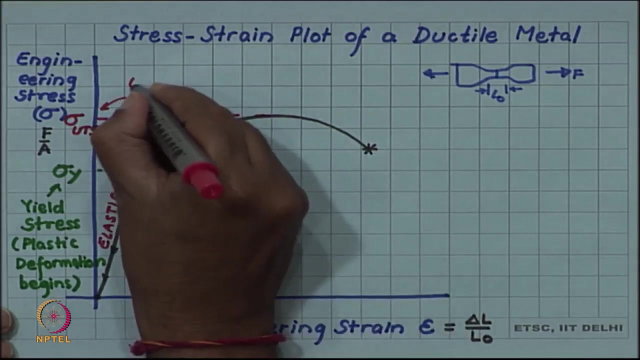 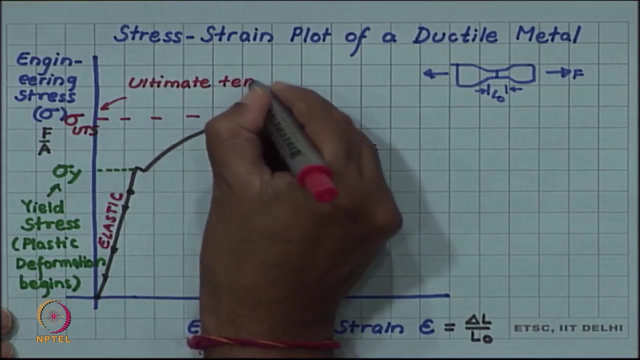 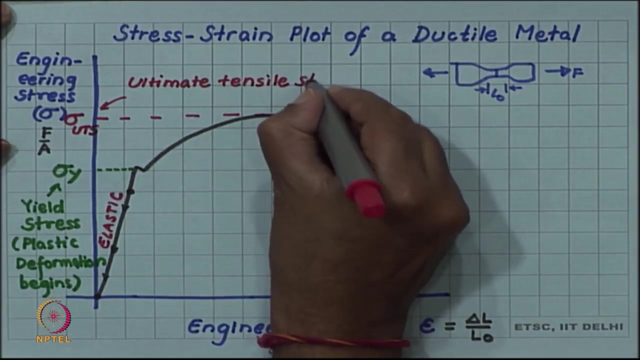 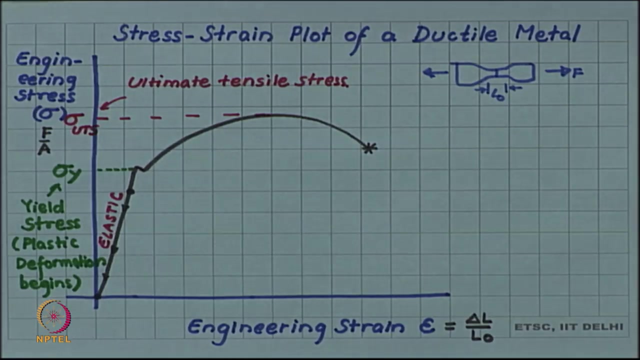 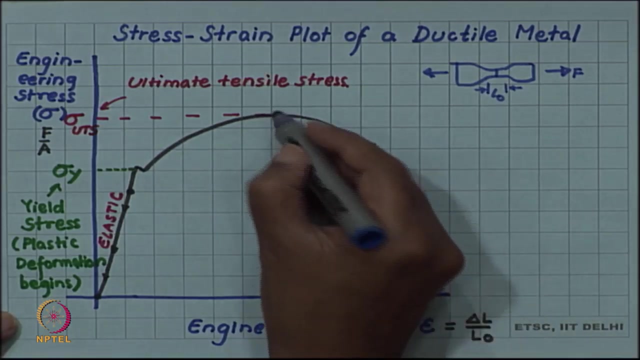 begins. Then the material reaches a sort of maximum load corresponding to the maximum point on the curve and the stress corresponding to that is called sigma U T S. That is ultimate tensile, The stress. and finally, after U T S, actually what happens? that material develops a neck. 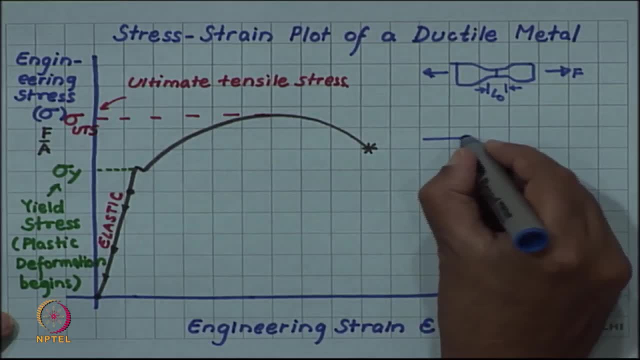 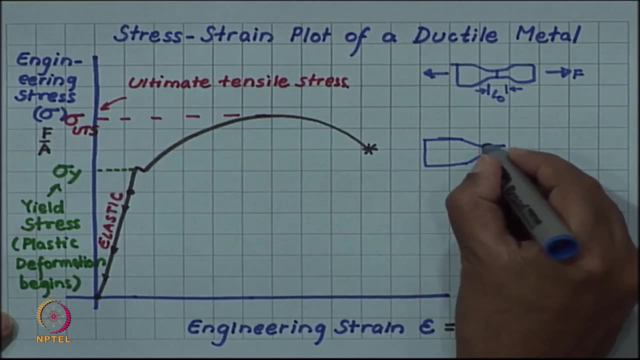 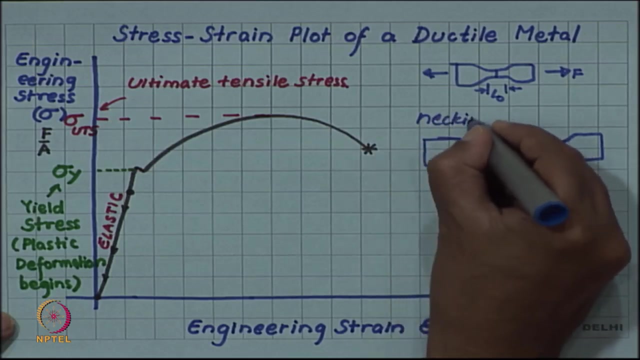 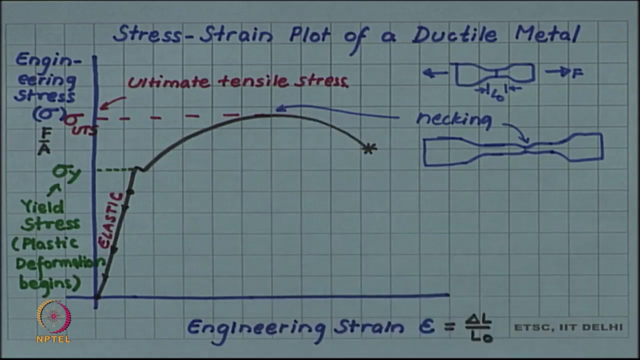 in its gage length. suppose this was the uniform gage length. But then suddenly, at some point it will develop a neck. this is called necking, That is, the cross sectional area is reduced at one given point. And this happens at this U T S point. the neck develops as soon as the neck develops. 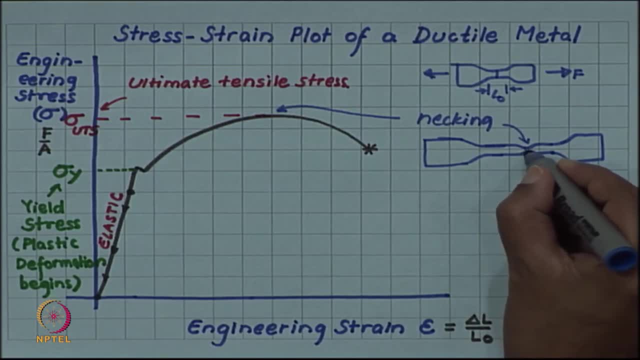 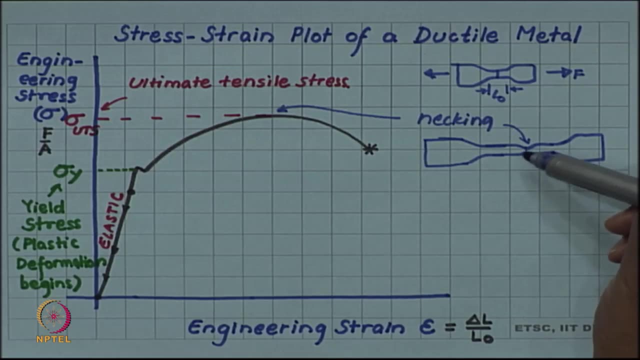 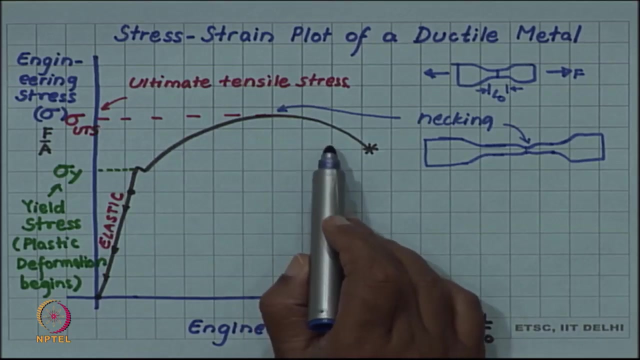 the further deformation is concentrated at that point because the cross sectional area reduces, So the stress at that point starts increasing and so more and more deformation is now concentrated there and further increase in the engineering stress is not required because the cross sectional area is decreasing. 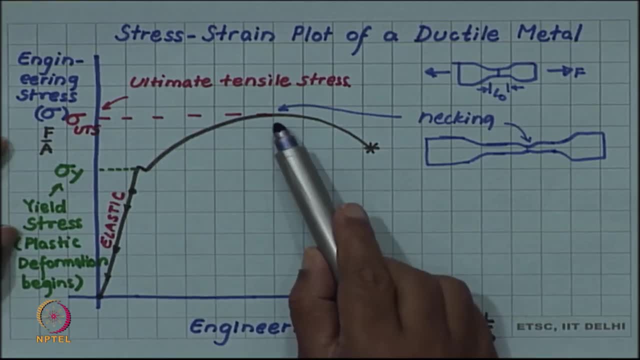 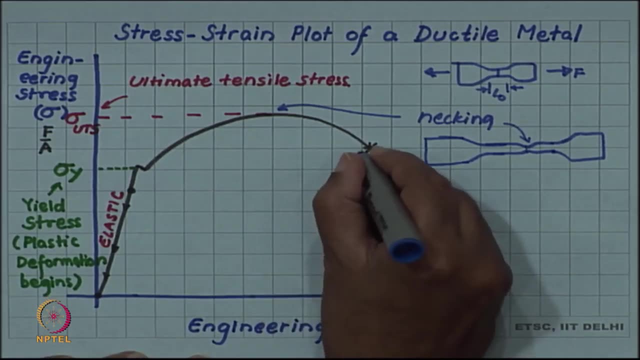 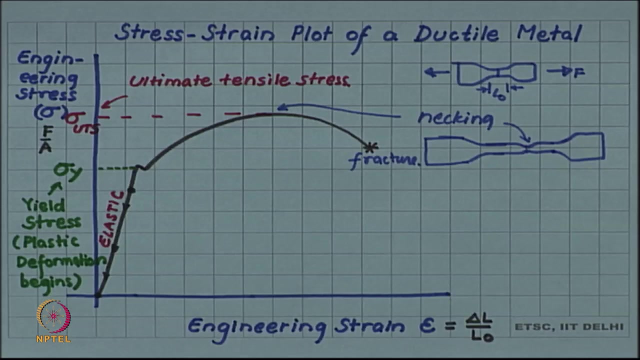 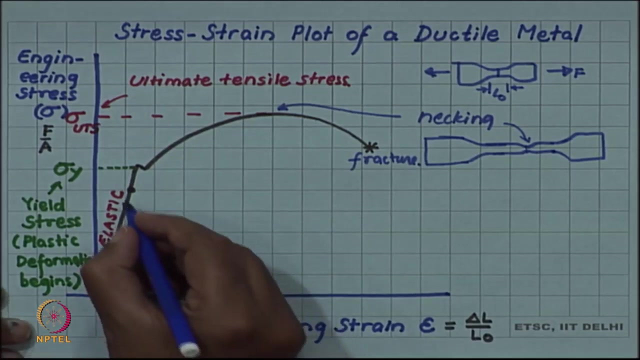 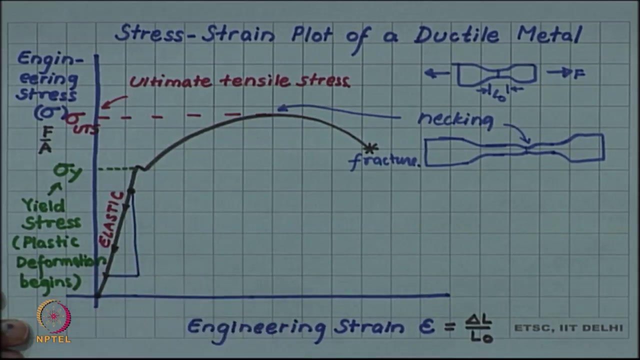 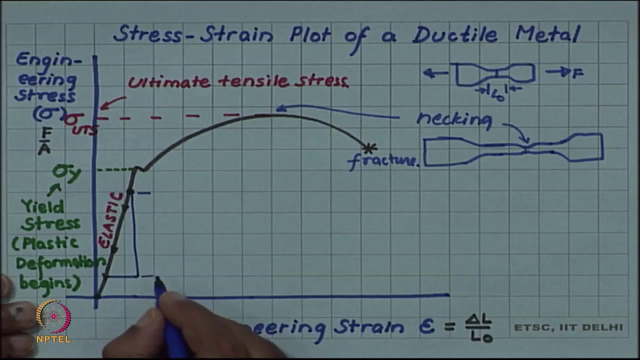 So even at a lower load, you still have quite high stress for deformation and the deformation progresses. and finally you have the fracture point. Now, if we look at the elastic portion and if we look at the slope of the elastic portion, the slope is less than 1, 0.. 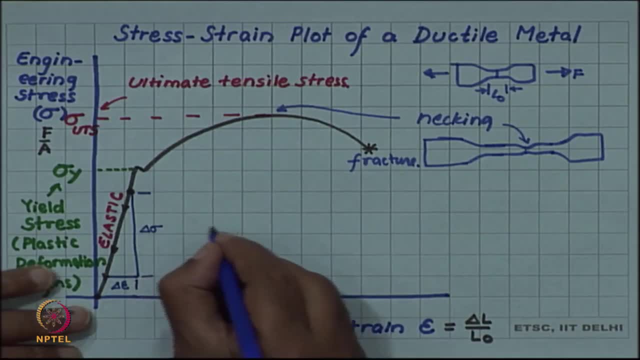 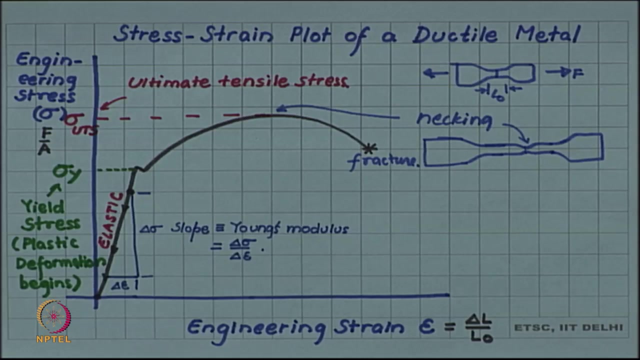 So this slope is known as the Young's modulus flow. This is a measure of stiffness of the material that higher will be the Young's modulus, more stress is required to create the same amount of strain. so this is called stiffness. and we also have a measure of ductility, which is, if we drop the perpendicular from here. 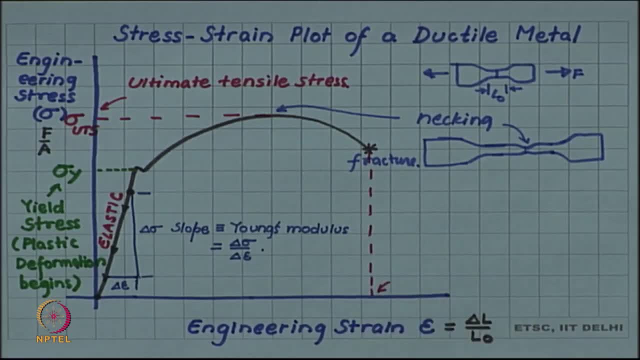 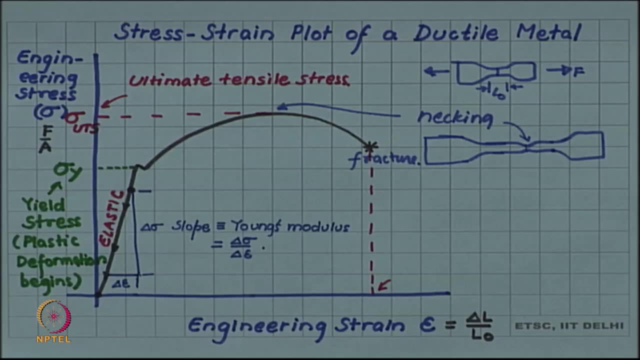 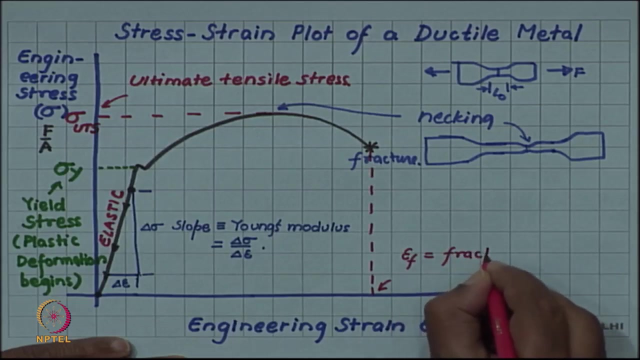 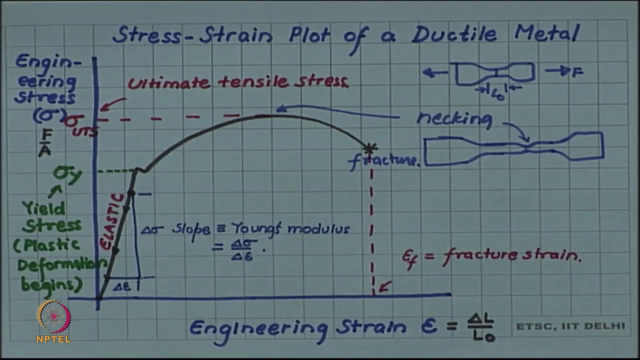 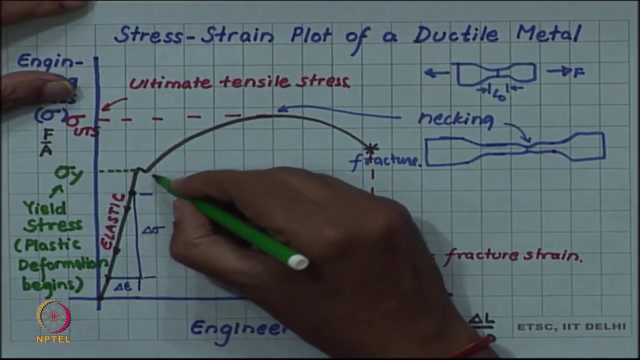 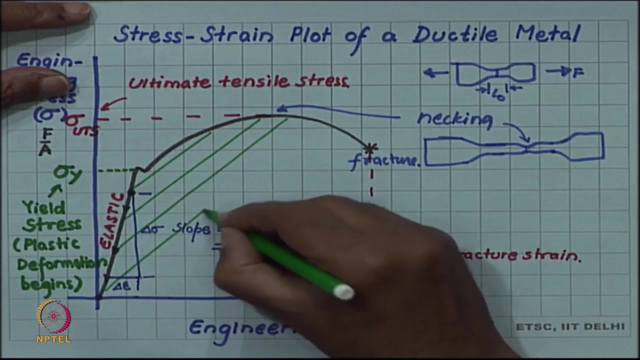 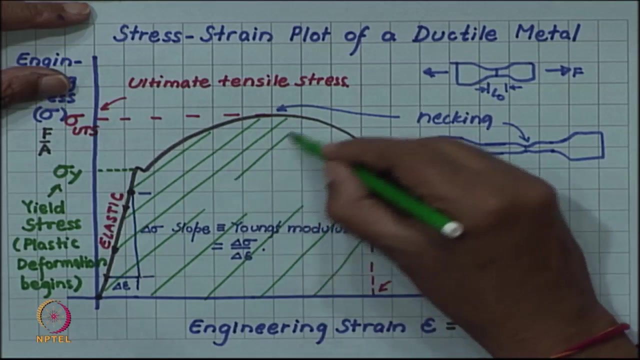 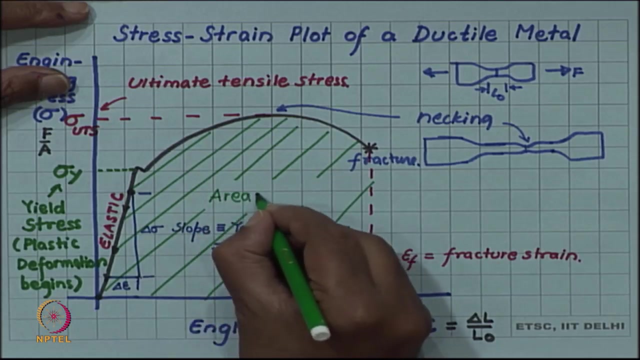 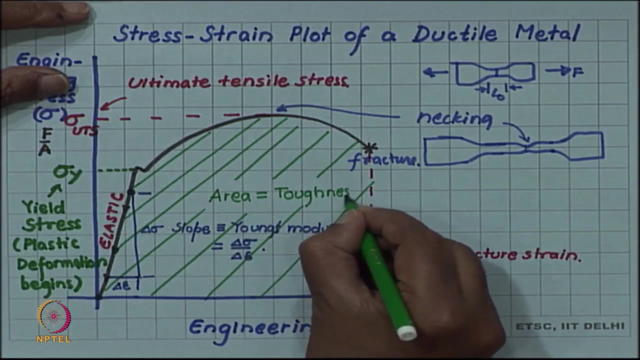 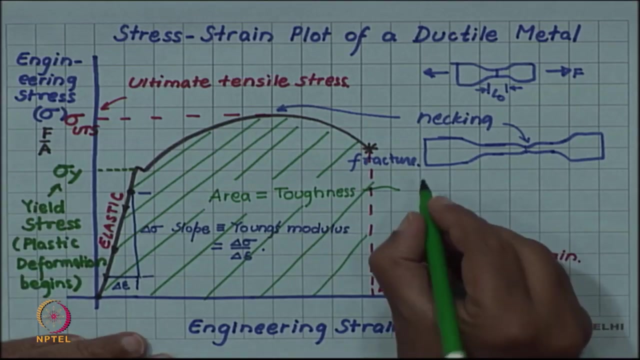 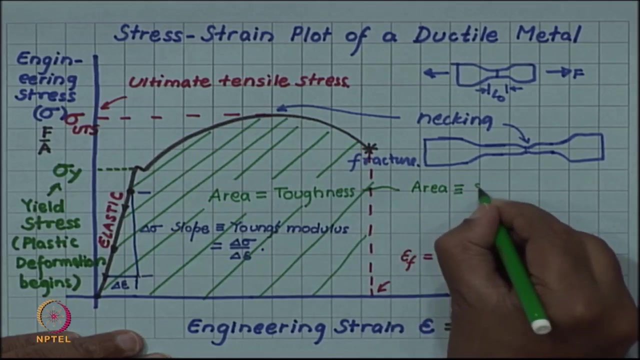 and get what is the strain at this point. That strain is the fracture strain. E, f is fracture strain. Now one can find the total area under the curve. this area in this is called toughness. Notice that since our axes are stress and strain, the area will be stress times, the 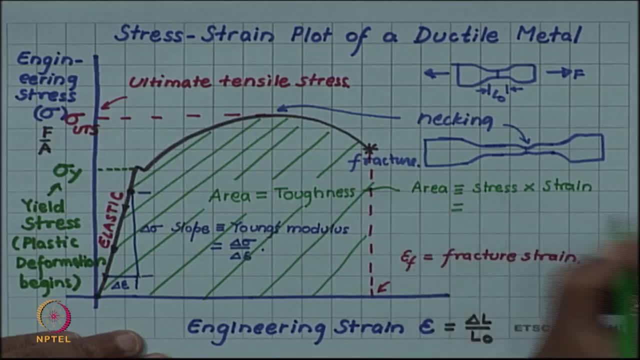 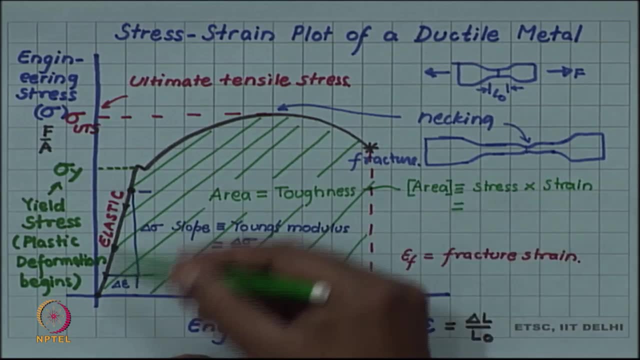 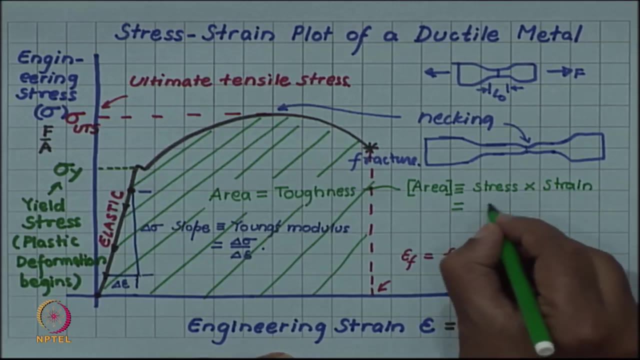 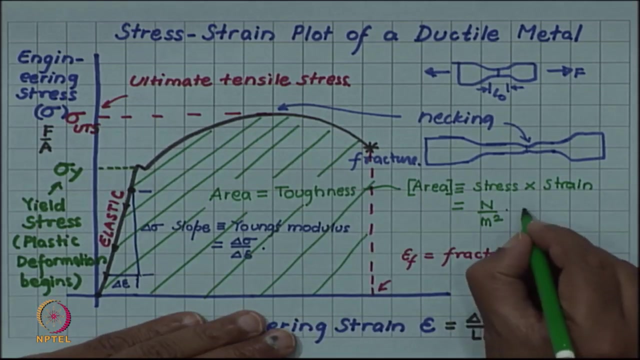 strain In terms of the units or dimensions. you have to actually integrate the area under this curve, So the dimensions will be stress times strain. the stress is in. you can think of it as Newton's per meter square and a strain is a dimension less quantity. So the dimension of this area is Newton per meter square. this 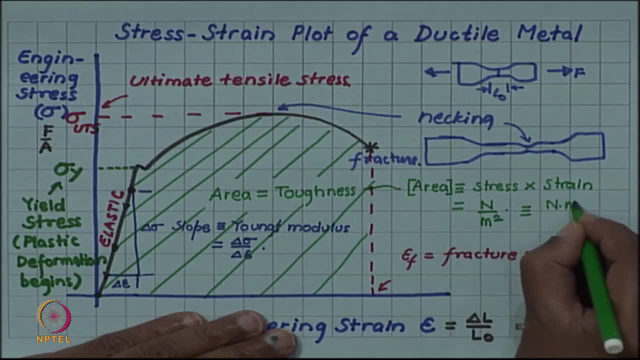 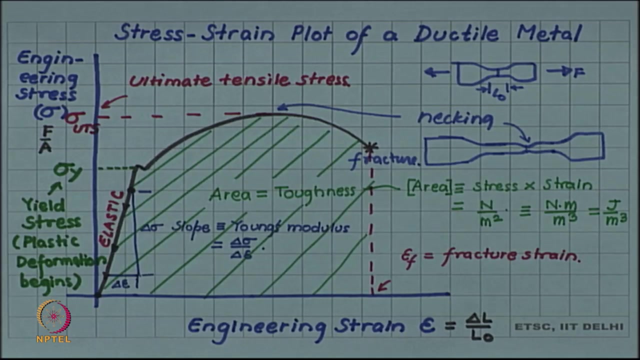 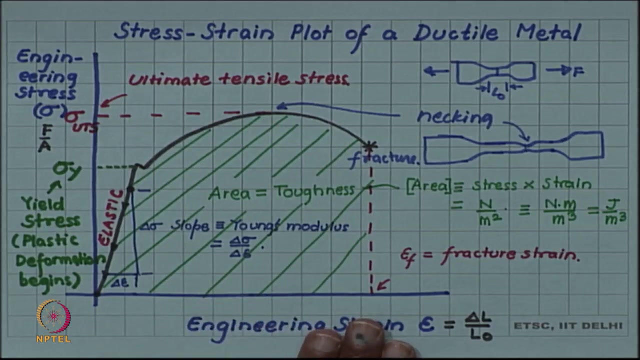 can be thought of as Newton, meter by meter cube or joules per meter cube. So this area is energy per unit volume which has to be provided to the material up to the point of fracture. So this much energy per unit volume is required to fracture the material. This 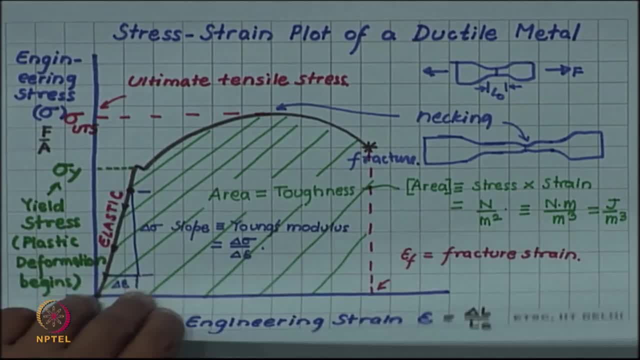 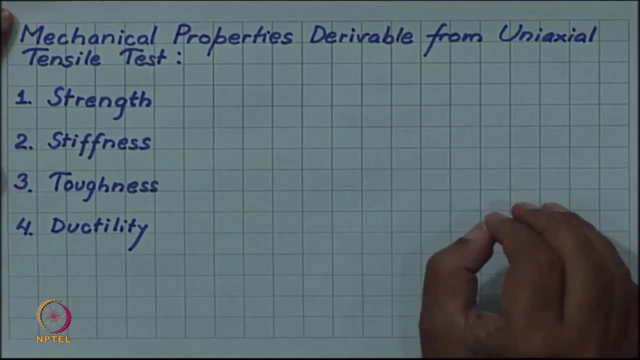 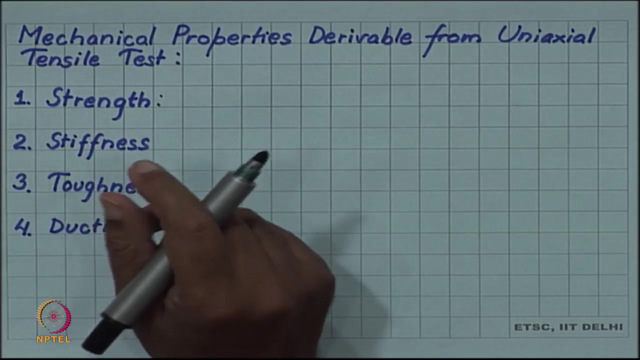 is called the toughness of the material. So let us look at all these properties and summarize that- mechanical properties, which are derivable from the uniaxial tensile test, is the strength property. The strength is the stress value, either the yield stress or 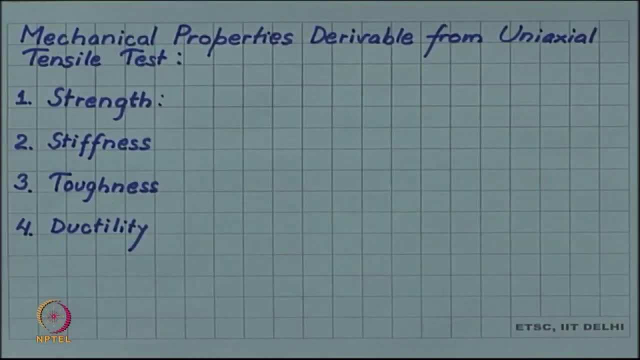 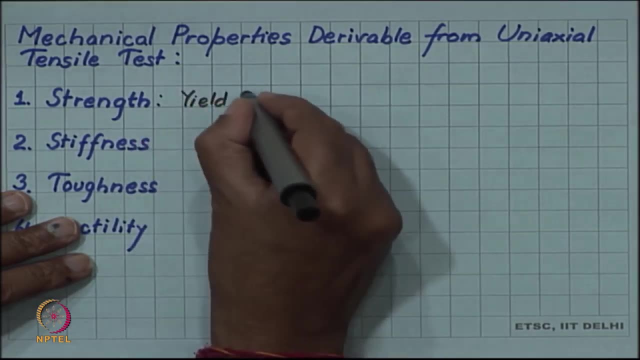 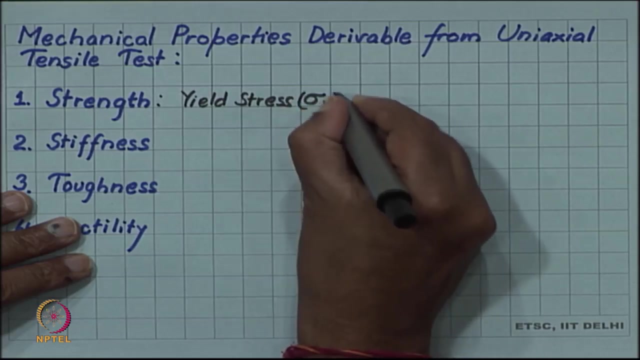 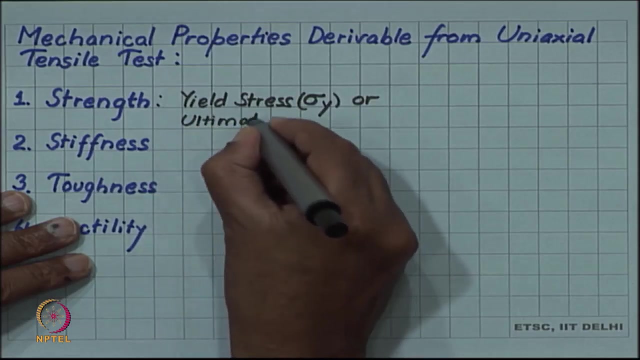 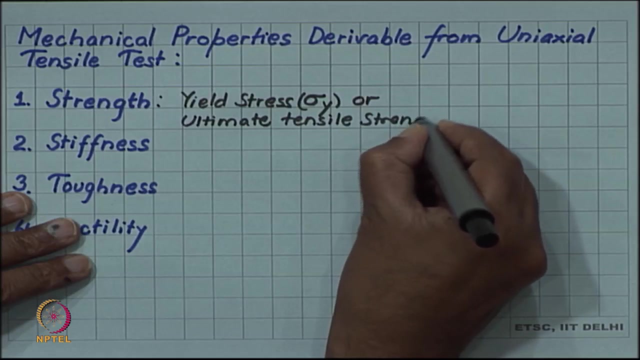 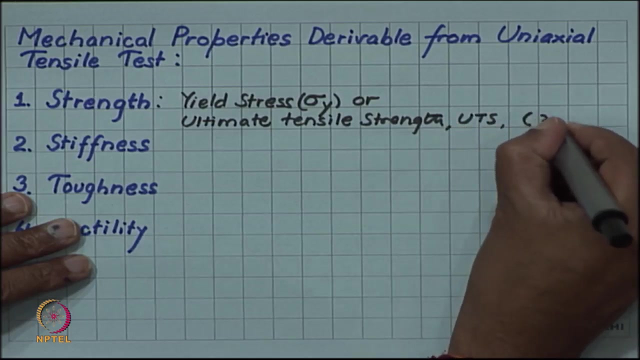 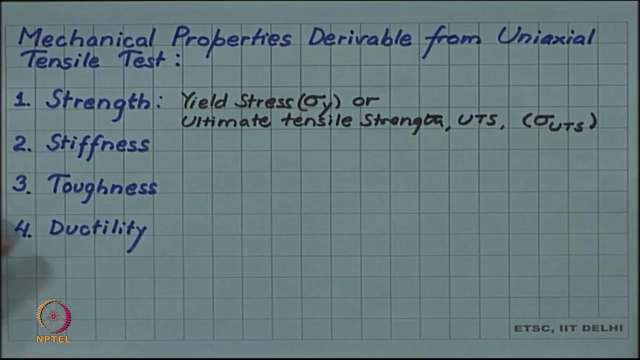 the ultimate tensile stress is considered to be the strength of the material. So So yield stress, sigma y, or ultimate tensile strength, also known as UTS. So this is the UTS, or written as sigma UTS. These two parameters are the strength parameters and they will. 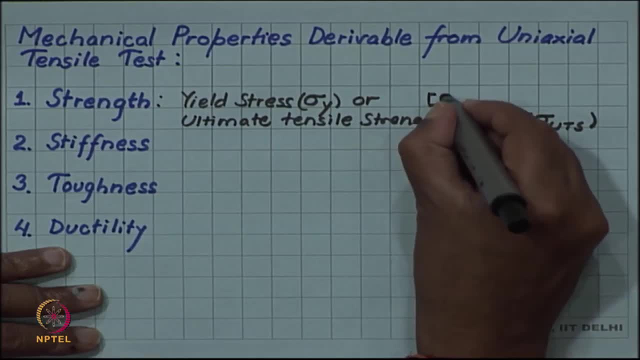 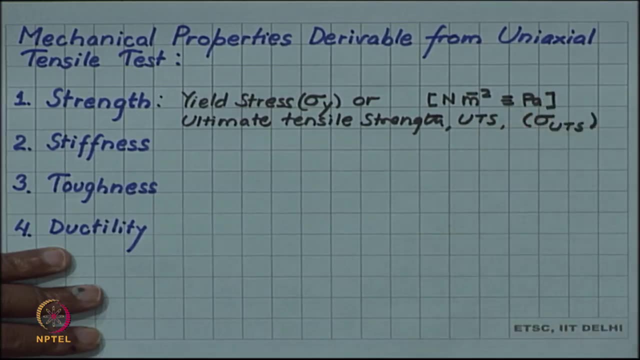 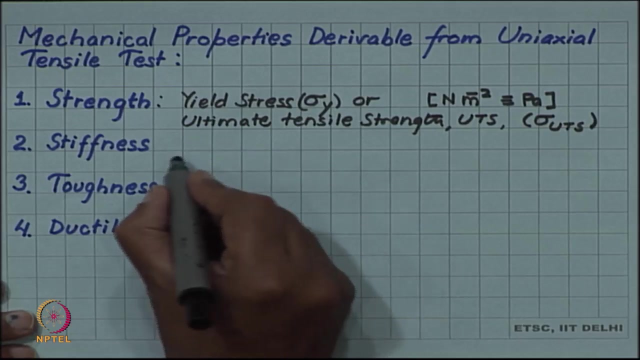 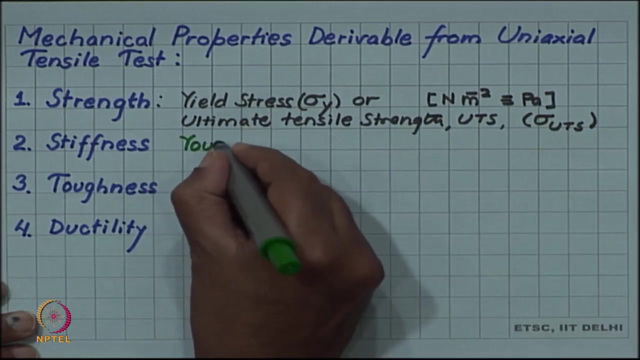 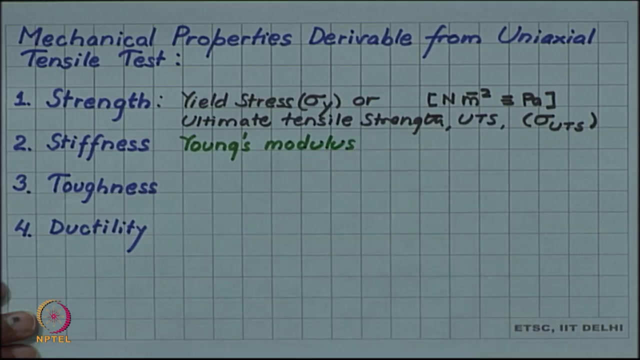 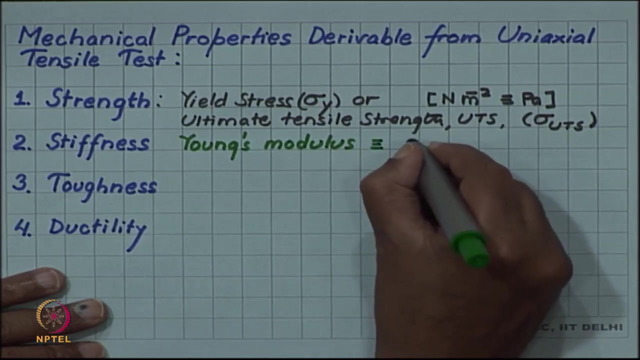 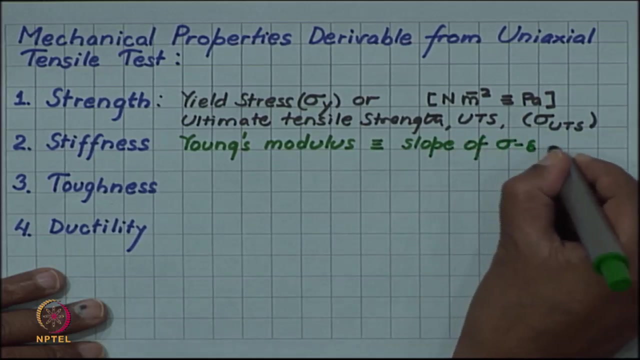 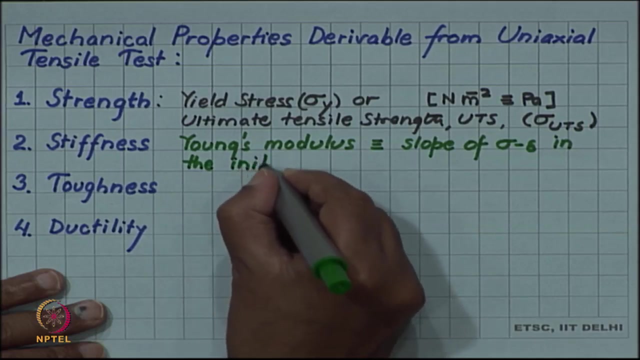 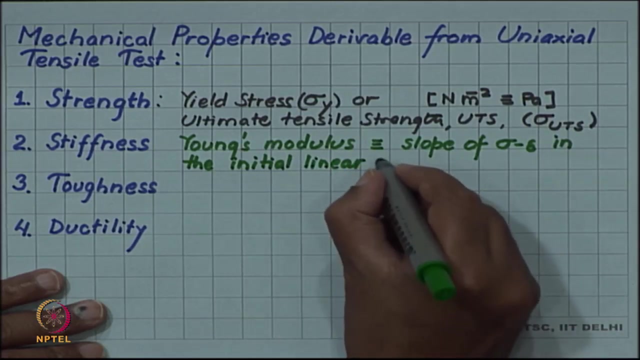 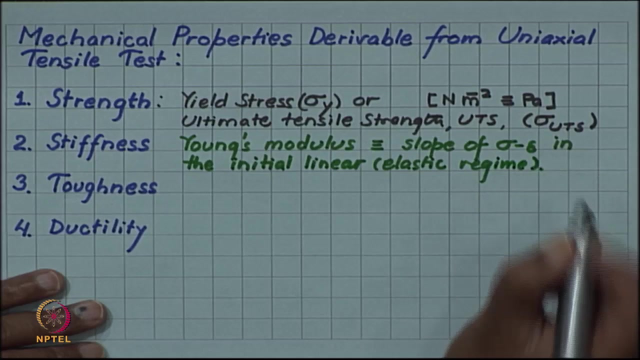 of course be measured in Newton per meter square or pascals. A stiffness of the material is given by the YoungÕs modulus and that is a slope of the stress strain curve in its linear part. loop of stress strain. linear or elastic regime. tight loop of stress strain. 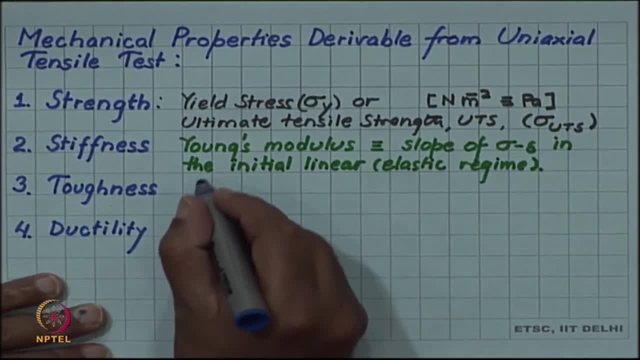 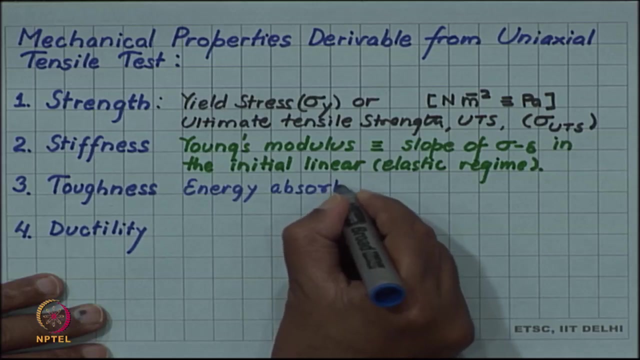 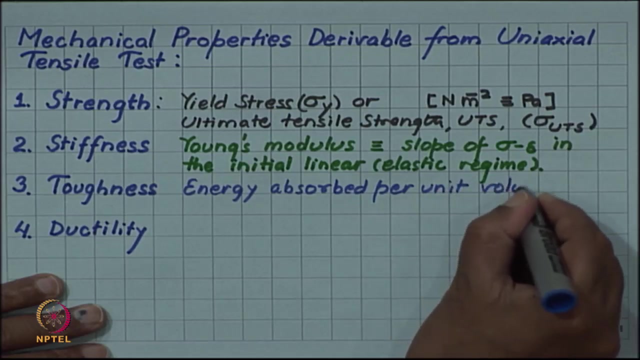 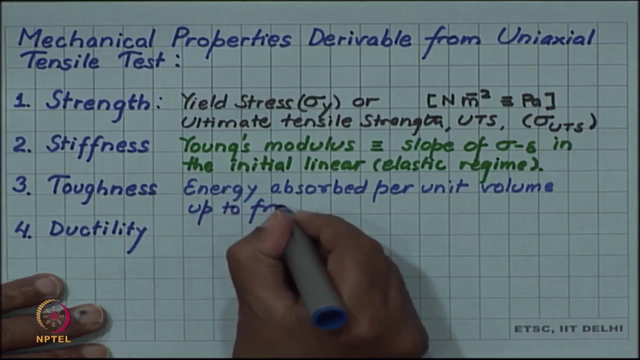 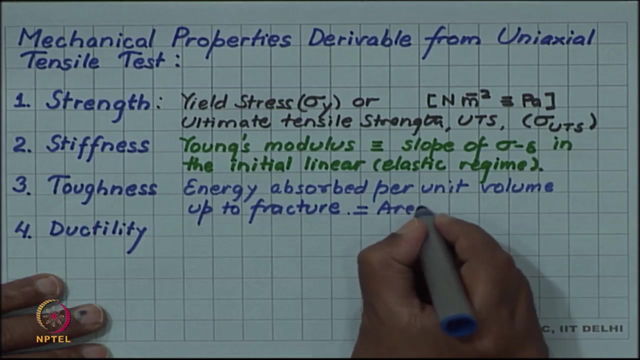 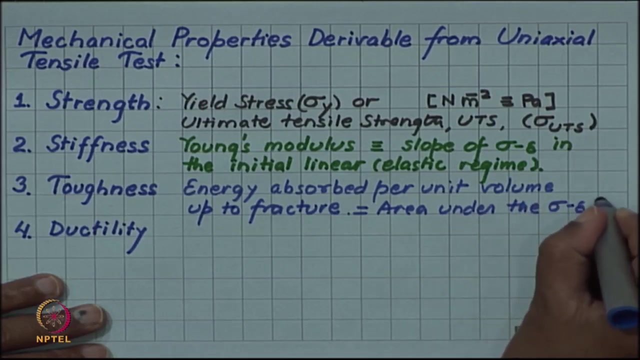 So toughness is property of material, that area under the curve. So energy absorbed per unit volume. So this is the area under stress strain plot. and finally, ductility is how much the material elongates. So the ductility is elongation up to fracture. 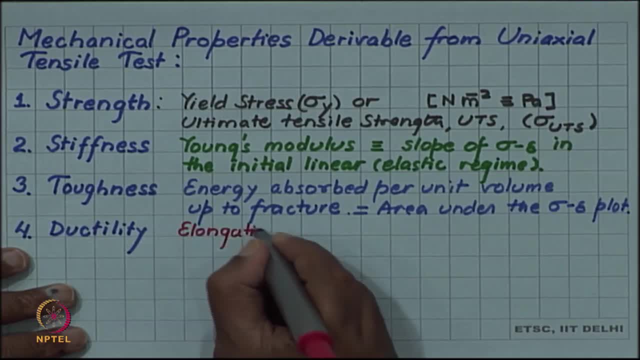 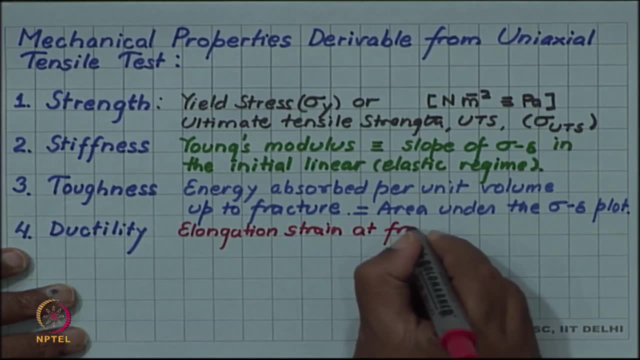 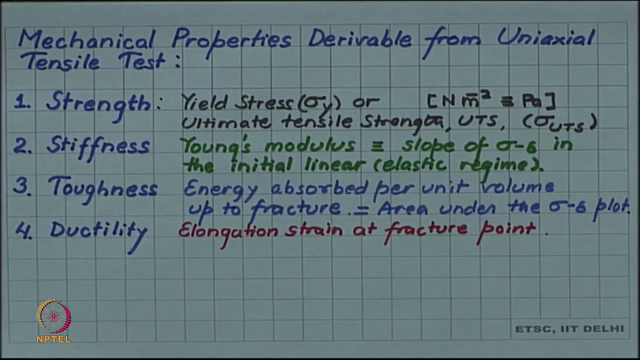 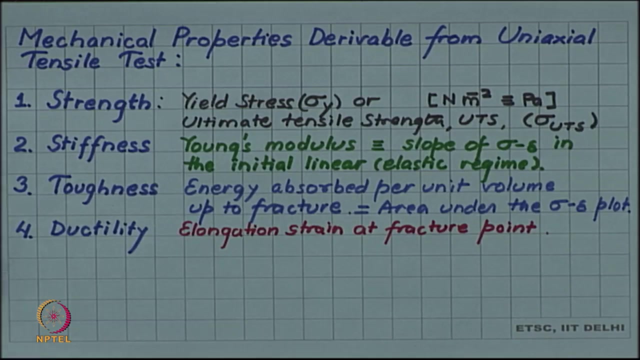 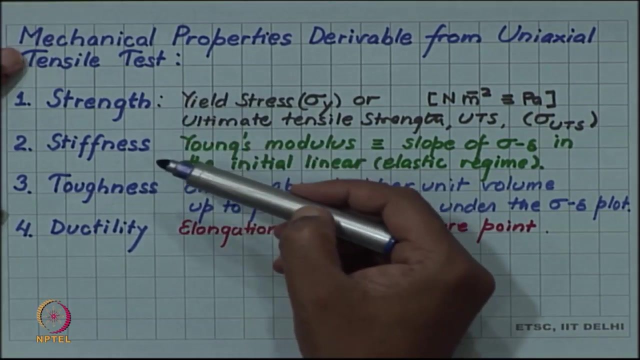 Elongation strain at fracture point. So notice that these different material parameter, which are easily derivable from a uniaxial tensile test, have different technical meanings and should be used in this particular sense, because in common uses strength, stiffness and toughness can sometimes be used interchangeably, but in